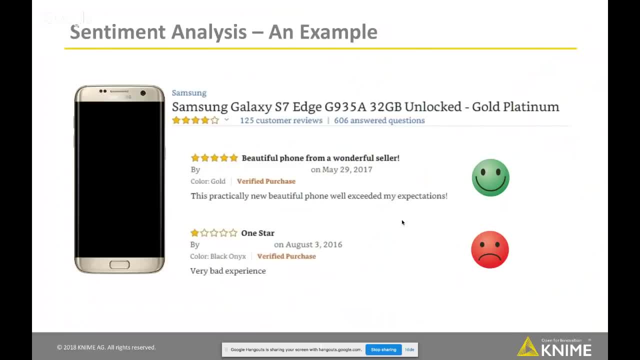 I look at some reviews, for example on Amazon, And for me as a person, it is often quite easy to understand whether a review is positive or negative, So I'm going to start with the negative. So, for example, this one beautiful phone from a wonderful seller is clearly positive. 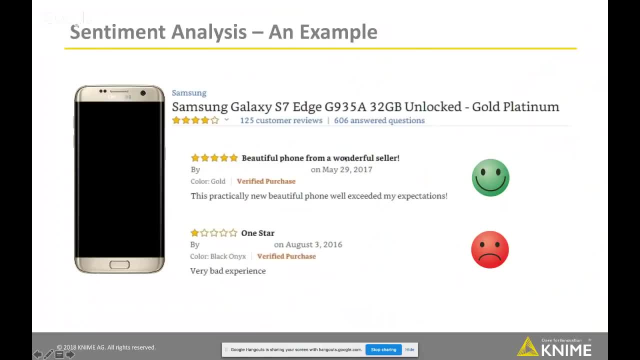 But for a machine it's already not that easy to extract from a text whether it's positive or negative. I myself I don't need an algorithm to analyze how many positive reviews are out there and how many negative reviews are out there, But for me, but if you are actually a manufacturer, 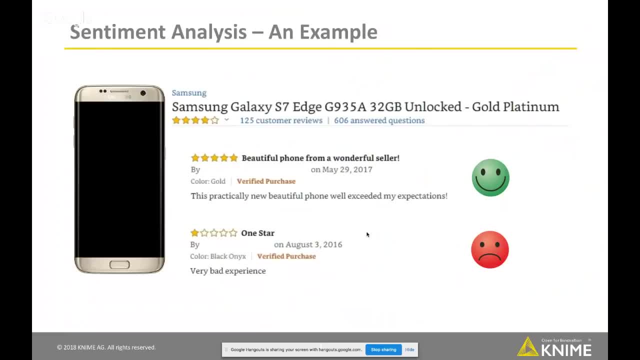 or you produce your phones. you actually you might be interested in these reviews as well, But you don't want to read them all manually. But you maybe want to catch all these reviews from the internet and analyze them automatically to gain some insight: what people like about your product and what people don't like about your. 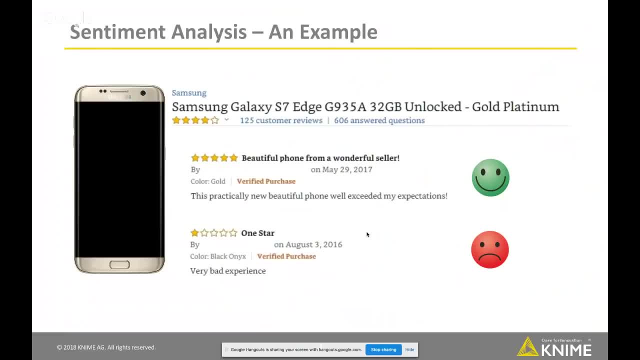 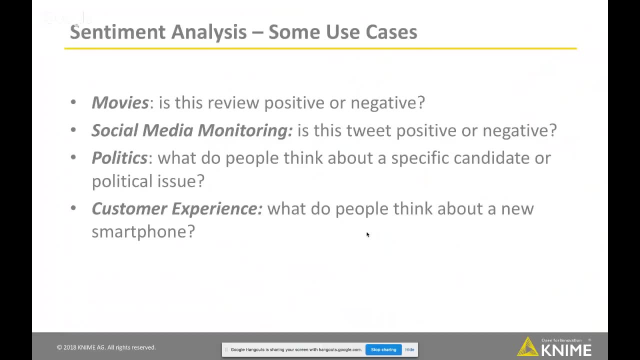 product. And this is only one use case of sentiment analysis. Other use cases for sentiment analysis is, for example, that you want to analyze movie reviews. this is also the topic we will take a look at today. so the use case for today is that we want to. 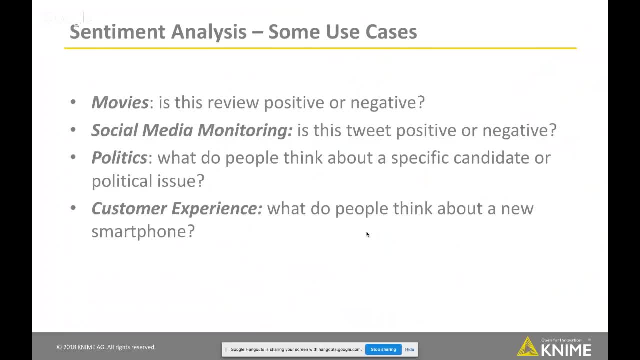 classify some movie reviews, whether they are positive or negative. another example is social media monitoring. so nowadays a lot of companies interact with their customers or leads via or via twitter. so you have a lot of tweets on twitter about your product and there it's also important maybe not only to know how many people tweet about you, but also how many. 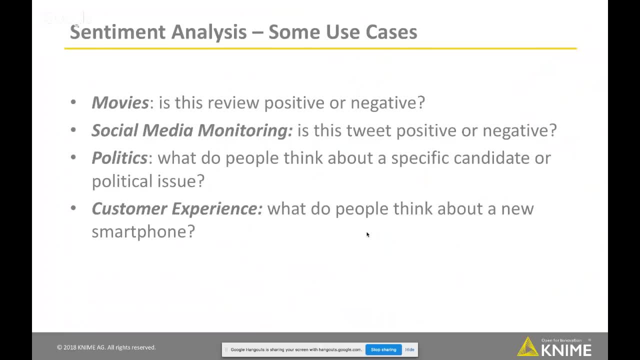 positive tweets and how many negative tweets do you get? and also, what is it what people like about your product, about your company or don't? another use case where you also can take into account social media monitoring is politics. so normally, before an election, you maybe want to analyze which candidate people do like or don't like, and 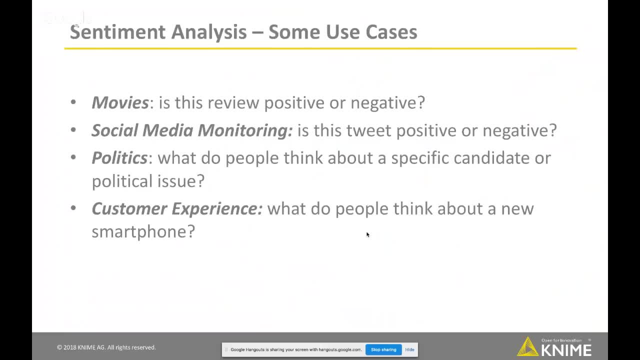 this is something that you can do by analyzing the tweet. so how many positive tweets do you get for a candidate or how many negative tweets do you get for a candidate, or not only before an election, but in general about political issues? what do people think positive about it or negative? and 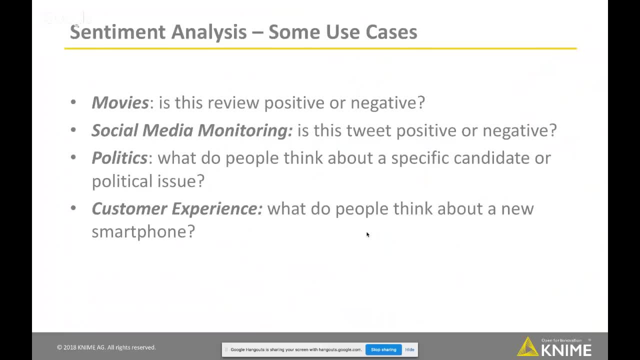 how many people post positive things about it and how many people post negative things about it. and another use case is customer experience in general. so with sentiment analysis you can find out what do people like about your product, for example about a new smartphone, or also what do 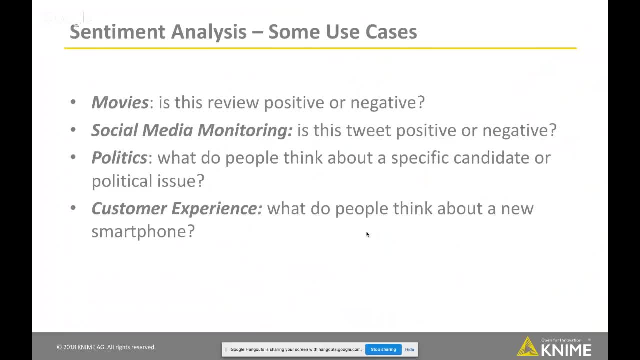 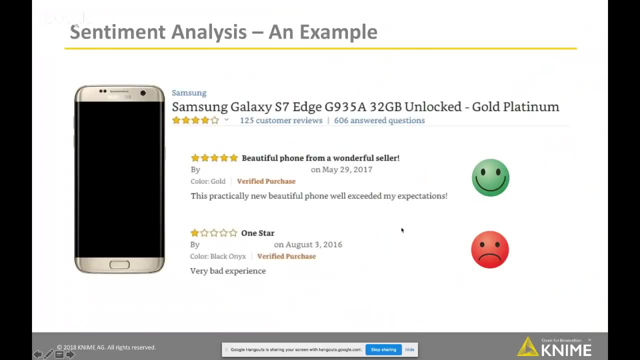 people like about your selling process? are they happy with it or are there things they don't like? in the two examples i did show here, it is pretty easy to understand whether it's positive or negative, because the positive review has words like beautiful or negative and the negative review 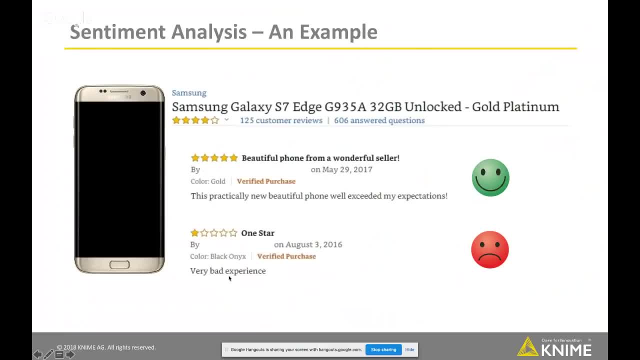 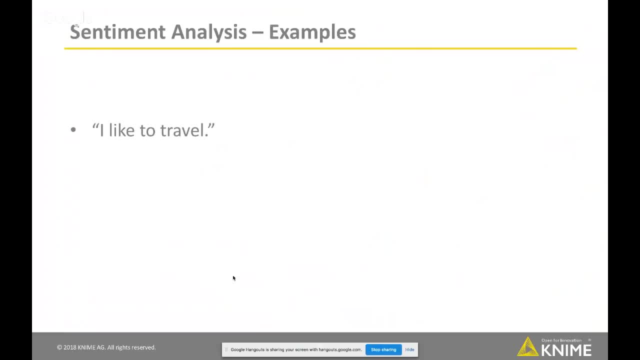 has words like beautiful or negative, and the positive review has words like beautiful or negative, and the negative review has words like beautiful or negative and the negative one has very bad experience. but actually language is much more complex. so if we take a look at the sentence i, 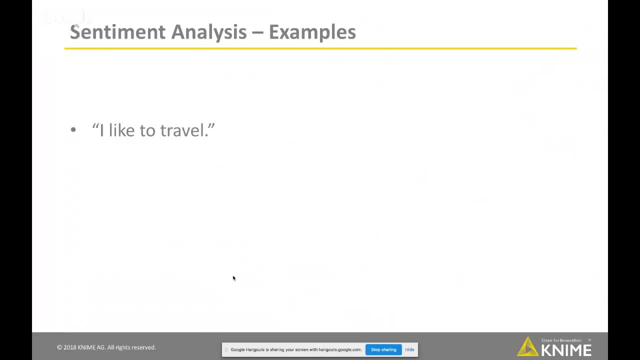 like to travel, it's clearly a positive um sentiment or it has clearly a positive sentiment. but if i add the word sometimes in the end, so i like to travel sometimes, this might be already not positive anymore, but even also not negative, but just neutral, and we both in both examples. 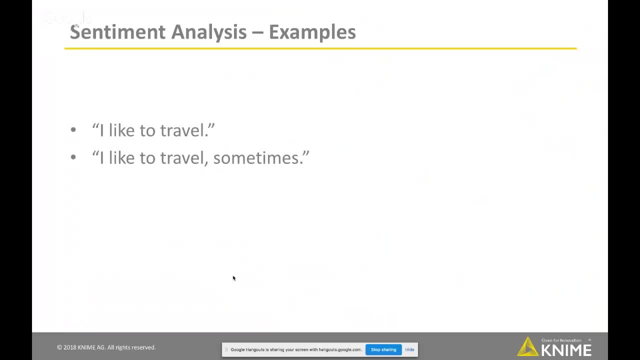 we have the word like. that tells us kind of the sentiment. and then it could be also that you have not dislike. for example in this sentence: i do not dislike cabin cruisers. so with a not you can make a positive word negative or a negative word like dislike, again positive, and then the language is: 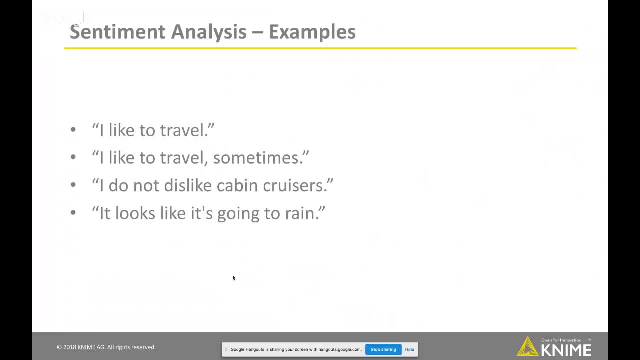 even more complex because, for example, the word like is on one hand a verb, when i say i like something, but it could be things like, be, also a preposition. like in the word, like in the sentence: it looks like it's going to rain there. it's not even having some meaning, which tells us something about the sentiment. 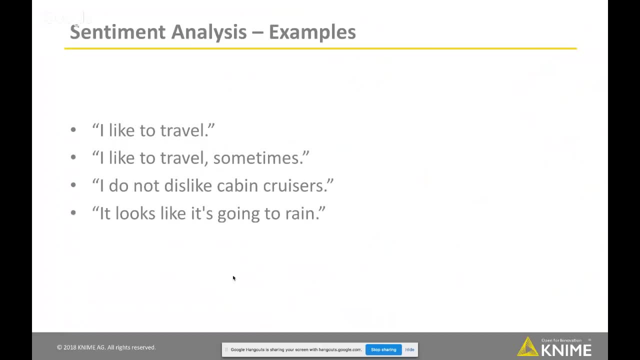 so you see this not as easy as it looked in the first place, if you want to extract the sentiment of a text. to summarize, what is the task of sentiment analysis, the task of sentiment analysis is that we want to train a machine or an algorithm to determine the expressed opinion in a document. 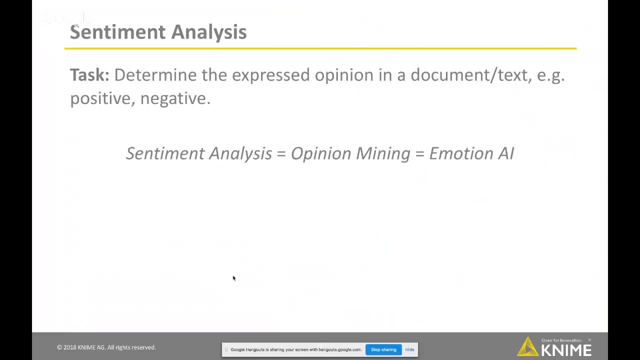 this can be, for example, whether it's positive or negative, but it could be also some other classes like really positive, neutral and really negative. those are the classic classes that you have in sentiment analysis, and sentiment analysis is often also called opinion mining or emotion ai. if i, if we talk about emotion ai, the class is: 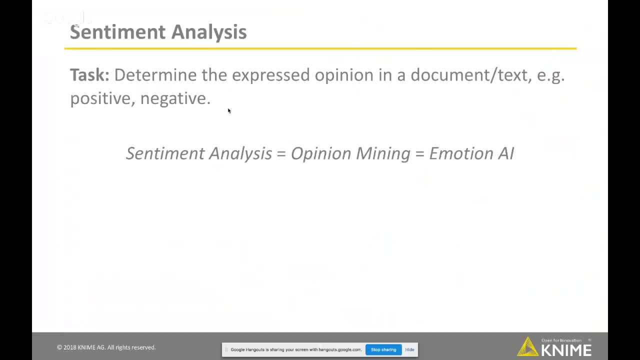 could be different. it could be things like happy or unhappy, but in the end it is really similar. the two approaches i want to introduce today is the first one, a lexicon-based approach, and the second one a machine learning based approach. in the lexicon-based approach, the idea is that 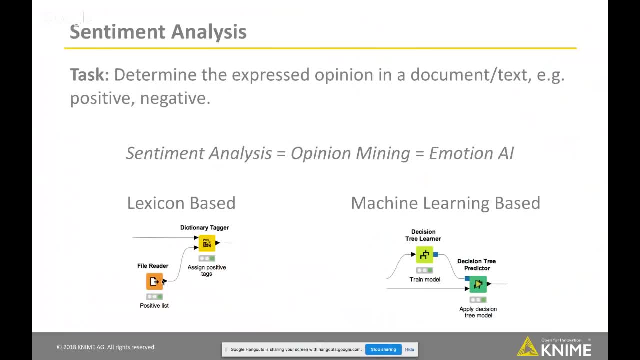 we use some manual defined rules to classify whether a review is positive or negative and in the machine learning based approach, we want to use some supervised learning algorithms that we can apply after some text pre-processing, when we have a numerical representation for each text, to actually train an algorithm which we can apply later and we here we will have a look at. 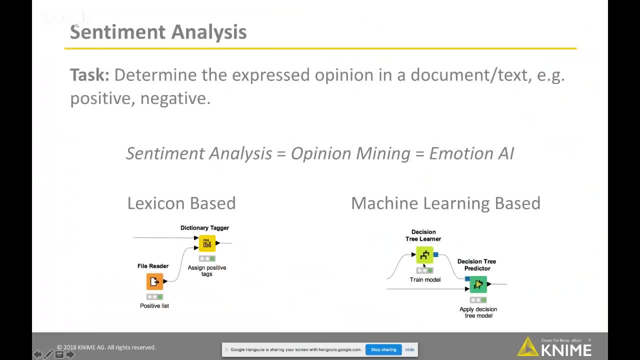 two use cases. on one hand, we will use some classic machine learning like the decision tree, and on the other hand, we will also have a look at a new name, keras integration, which is a deep learning integration in nine. before we take a look at the two different workflows, 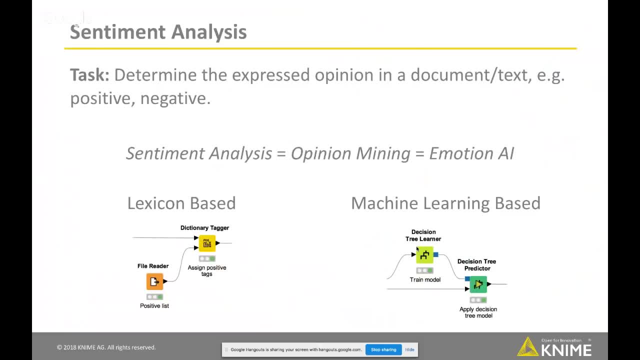 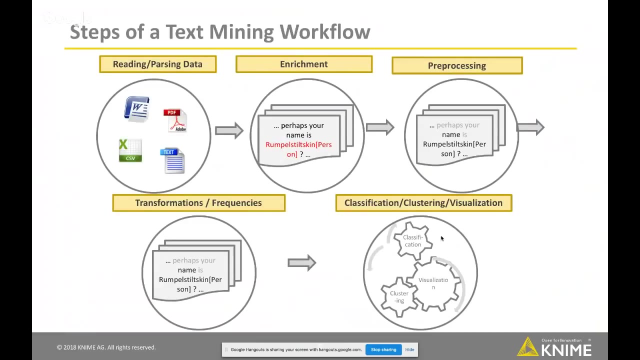 i will useiotable as a flieshow. the first one is a sensory assessment. so if you look at a sentence, I want to seeing the national advertising data and, as you're successful or you know we're doing good work and i feel well-paid, I happy or bad. see that the among the year data science proving the same several times. so i want to take a look at the machine learning based approach and talk a little bit about the different steps in a text mining project in general, because those or the example of sentiment analysis is one example of text mining and in the text mining projects we have always kind of the same steps. 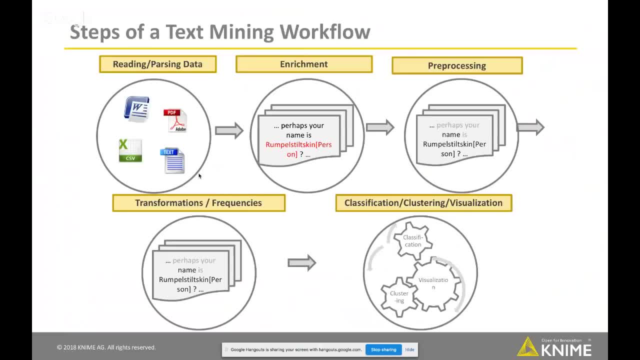 to either read a CSV file or a TXT file and then convert it to a document, or use, for example, the Tikka parser node to read a PDF and then have it already in document format. And document format for those of you who haven't worked with the KNIME text mining extension: 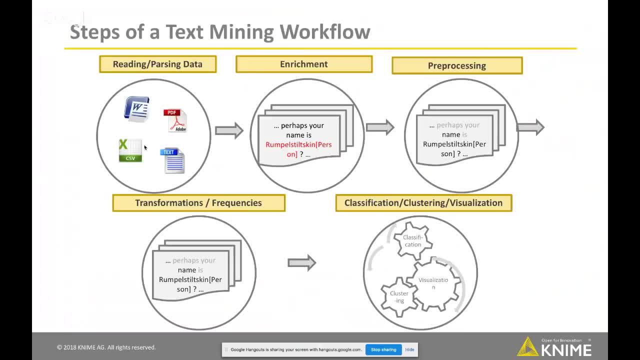 it's a special data type in KNIME, how we handle documents, And I will talk a little bit more about it during a small demo. The next step is then the enrichment part, And in the enrichment part we want to add additional information to our documents. 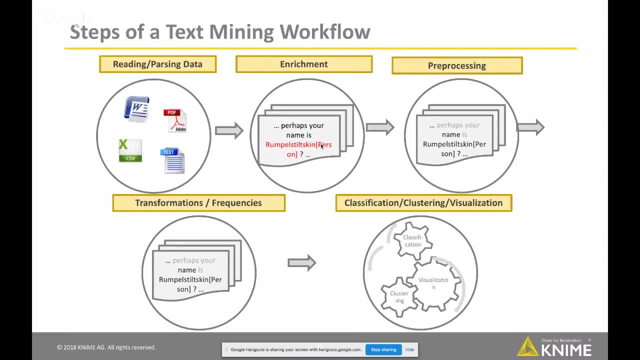 by adding tags to the different words in the document And tags you can see them as stickers that you add to each word, and there you have different tag types, for example, part of speech tags that you would assign to each word, whether it's a verb, a noun and so on. 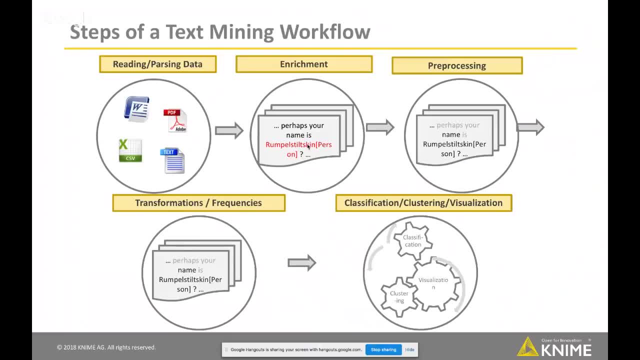 Or we can have also dictionary tags, what we will use later to assign tags like text, which we don't use that often positive and negative. The next comes the pre-processing step And in the pre-processing steps we delete all the words that we don't want to take. 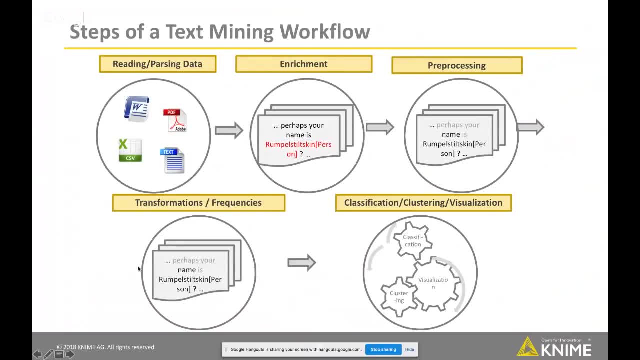 into account in our analysis. And last, we create a numerical representation for each document. And here we have again different options and we will see three different options actually today, in the three different approaches And, once we have done, a numerical representation for each of our documents. 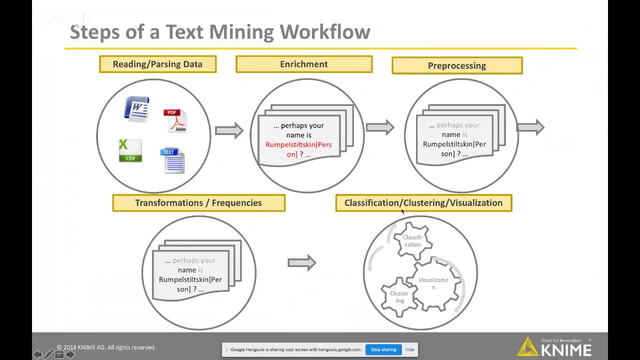 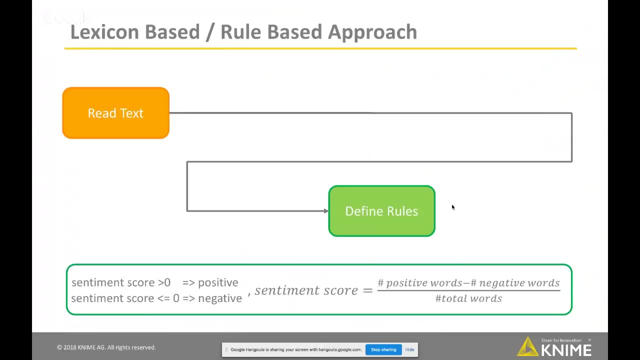 we can use all the classic nodes in KNIME to do classification, as sentiment analysis is in the end a classification problem, or also clustering or some visualization. So first we want to have a look now at the lexicon-based approach, which is also often called a rule-based approach. 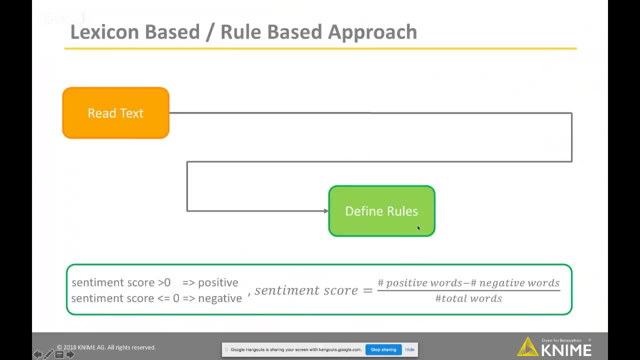 because we read in the text and then we want to define a rule based on which we decide whether a document is a review or a document has a positive meaning or a negative. The rule I want to define is that if I calculate a sentiment score, 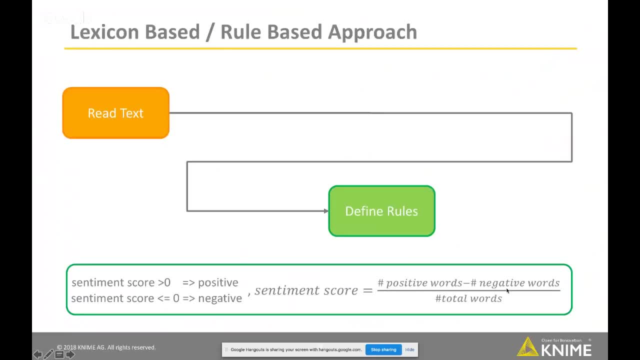 where I compare whether I have more positive or negative words and then I divide by the total number of words And if this sentiment score is positive, so we have more positive words in our document, I assign the class positive And if the sentiment score 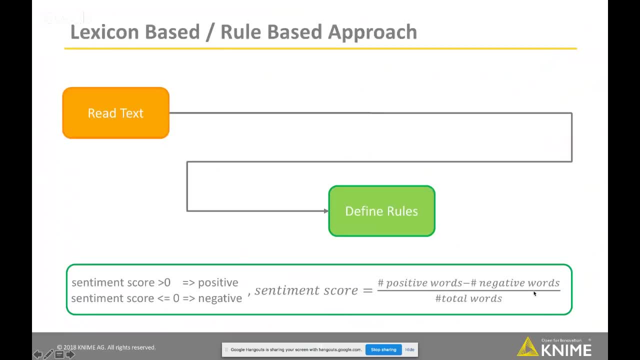 is negative. what would mean that we have more negative words in our document? then I want to assign the class negative. To actually calculate the sentiment score, I need to know how many positive words I have in a document and how many negative words I have in a document. 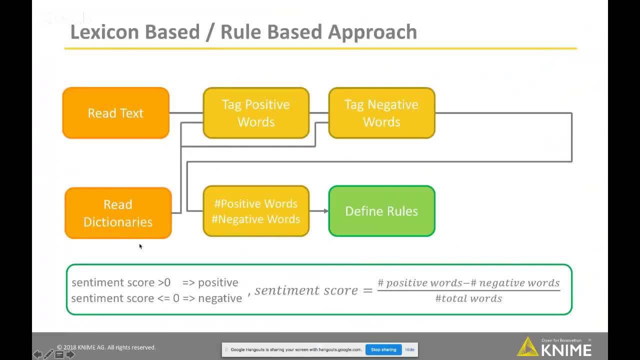 And to do so I read in additional dictionaries with positive and negative words, So one dictionary for positive words and one list or dictionary of negative words. And then I take the documents, or I take the positive and the negative words in my documents with two tag dictionary, tagging notes. 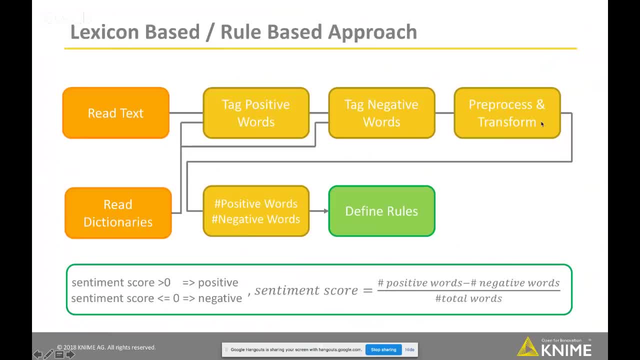 And then I do some pre-processing to actually delete all the words which I didn't tag, And once we have done this part- so we have now our finished rules- we can actually also evaluate how good our rule-based approach did work. And now I will switch to the NIME Analytics platform. 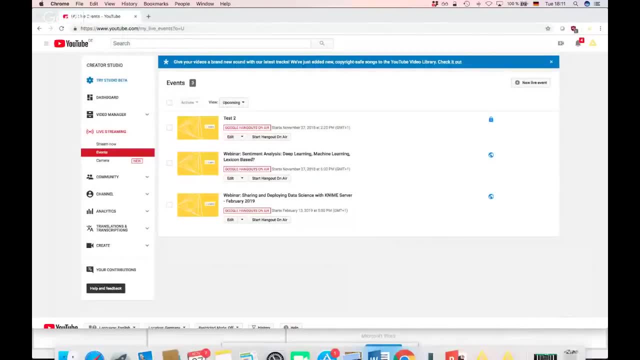 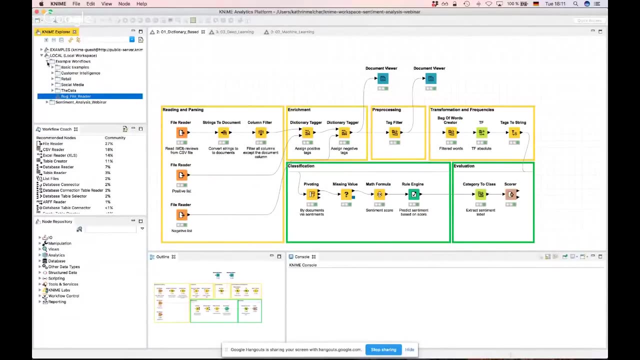 where I have this workflow open. So let's see here. So here we see a workflow which performs exactly this, this task. So here we read in the different documents, which is, on one hand, the IMDB reviews, and then here the list of positive and negative words. 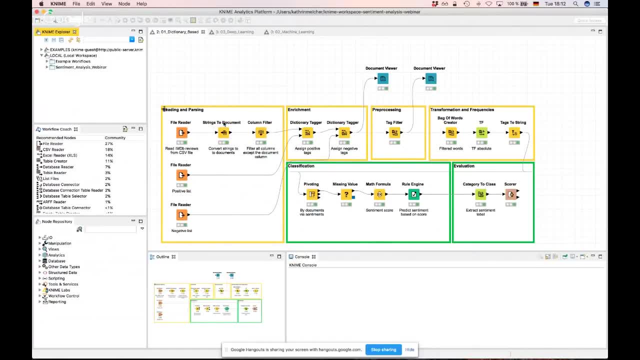 Then the first thing I do is that I create this document cell, which is this additional data type which we have in NIME, And in this document cell you can then have on one hand the text, but in addition also additional information like the author, the title or the category. 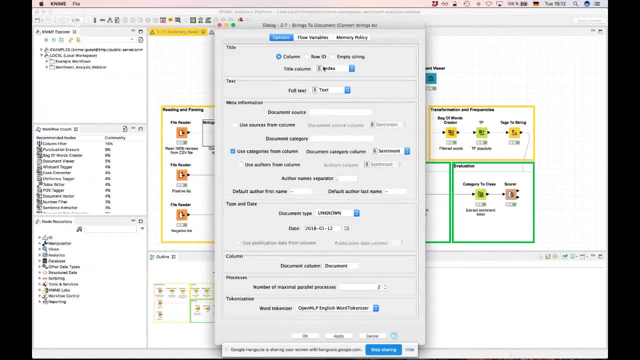 So if I double click the node and I go to the configuration window, I can select in which column I have: the index, the title, the full text or also the category information- in our case the sentiment- And then, if I look at the output data, I can also see that the text is selected and the summary. So that means that when I get a comment, if I want to create a summary, I can do this really fast. So that is just one simple step And then, once I complete this, I can actually do it in the next step. 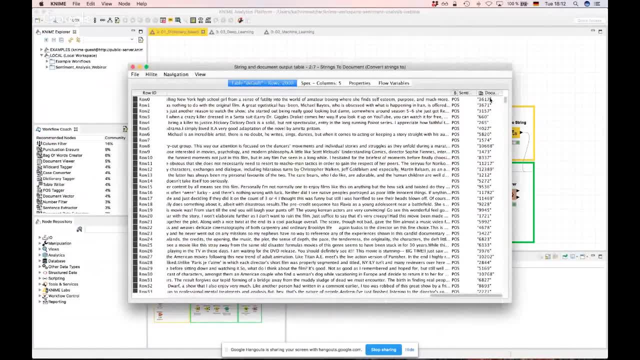 and I go to the right. I see here I have this document cells and in this document cell I see now here only the title where I use the index, but actually in the cell I have all the information which I see here, like the text and the category. 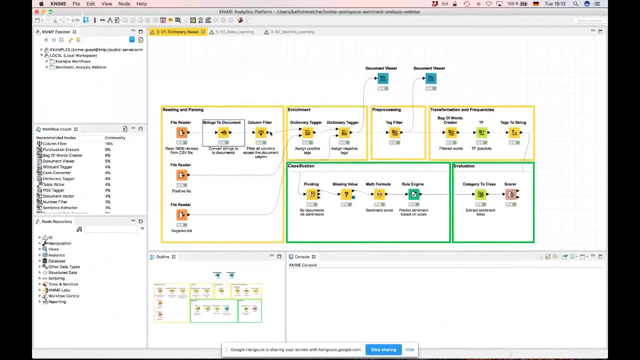 So I can delete these columns again, as I have all this information now in the document cell and I don't need them for now. Then, as I said, we want to tag the words with the positive and the negative tags and therefore we can use two dictionary tagger node. 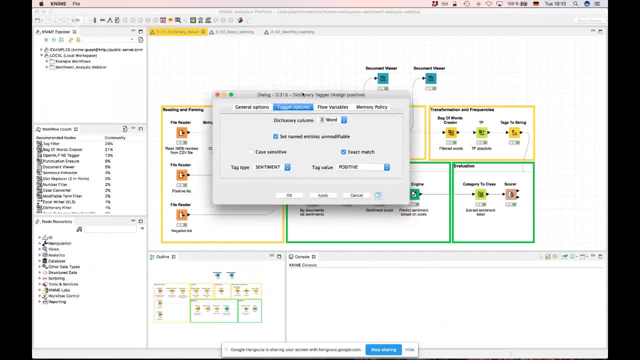 And if I go now into the configuration window of the dictionary tagger node, I see I can define here in which column I actually have my positive or negative words- in this case the positive words- and then I can define a tag type and a tag value. 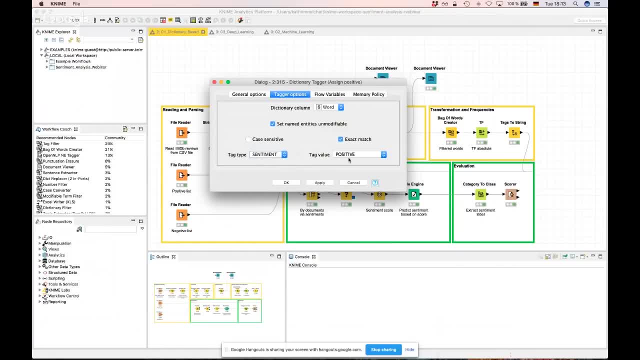 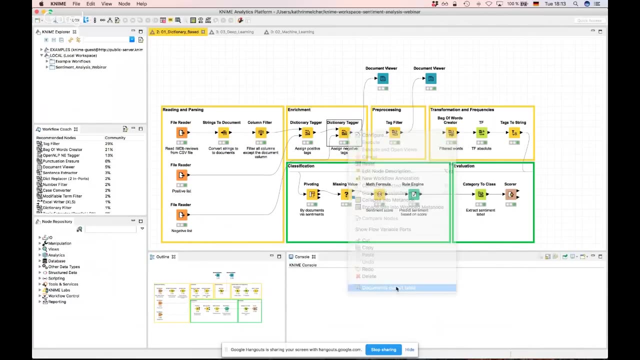 The tag type in our case is sentiment, and as we use the positive word list, we say the tag value should be positive And I can say okay, And here I do the same for the negative tags. Now, if you look at the output table, 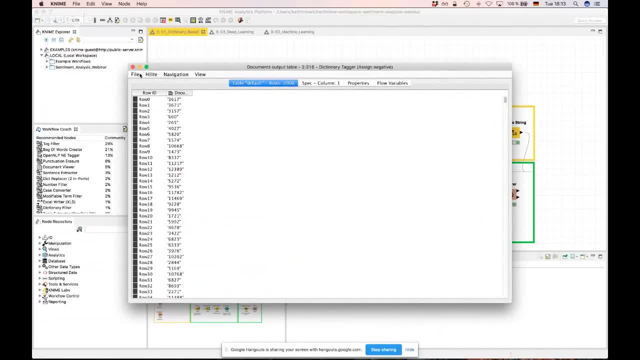 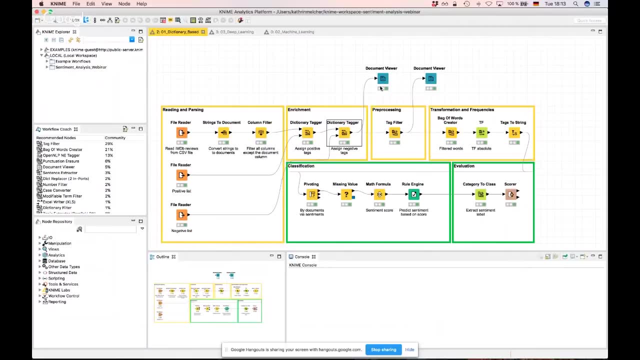 it looks like nothing has changed. We still have only our documents in here, but with the document viewer node we can actually take a look how the documents or which information is in this document cell. So if we right click on the document viewer node, 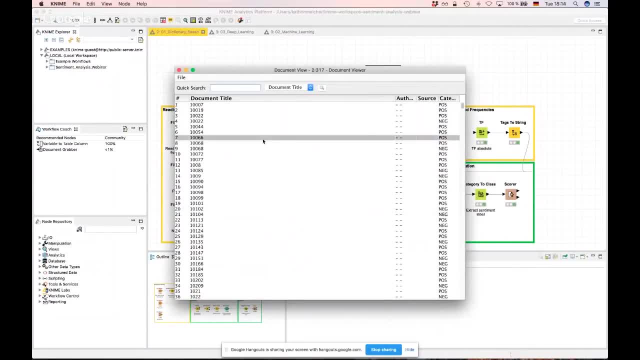 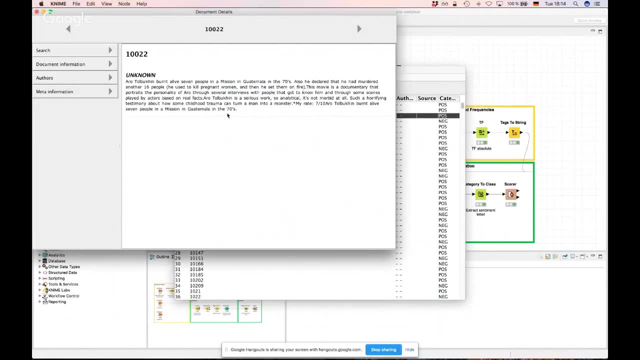 and we say view, document, view. we see here a list of all the top documents And the title, in our case the index, And if I double click now on one, I see here the review, And in here I can now also visualize the tags. 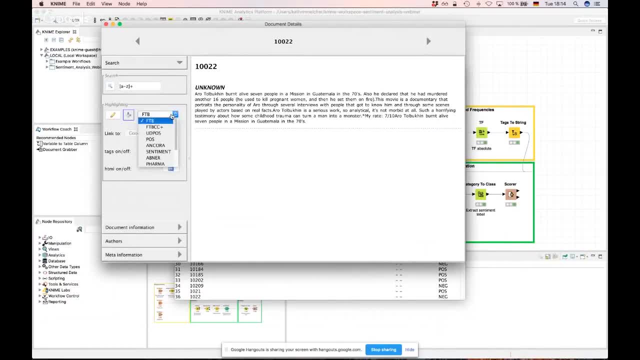 And to visualize the tags I can click on search and then select here the tag type- in our case sentiment- and then say tags on, And now I would see all the tags. So, for example, the word kill got tagged with the tag value negative. 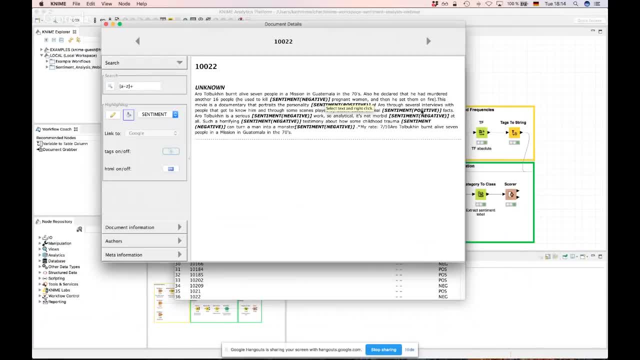 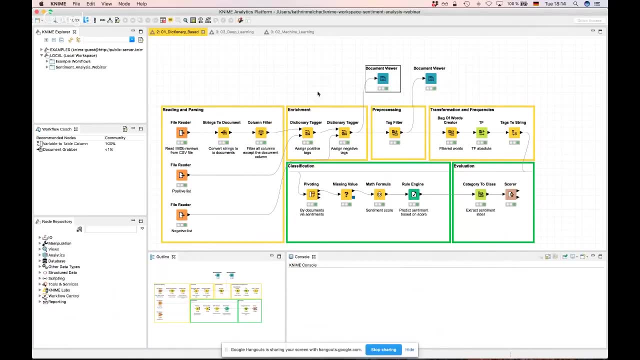 And, for example, reel got a positive tag. So and with the tagging, we are actually done already with the enrichment part in the rule based approach And in the pre-processing part, the only delete all the words which we didn't tag. 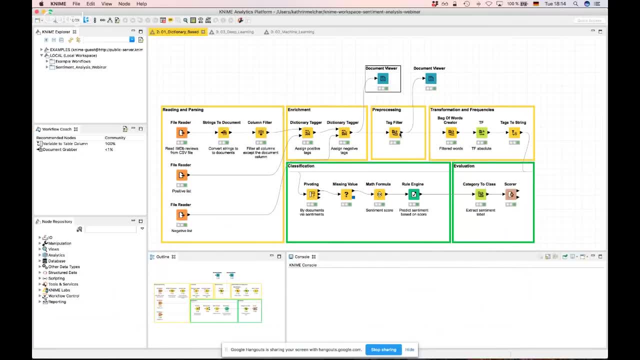 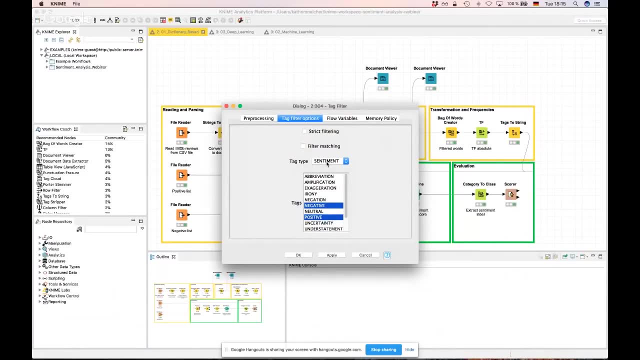 because for the rule we need only the words which got either a positive or an negative tag. So in the configuration window I can say: okay, I want to filter based on the tag type- sentiment- and I want to have only the words. 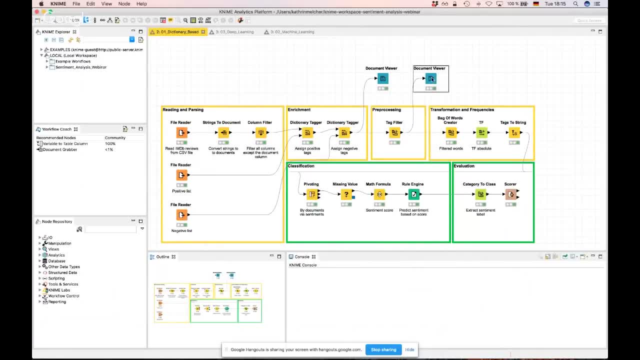 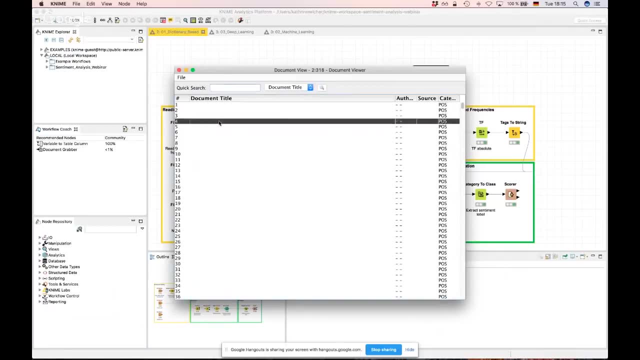 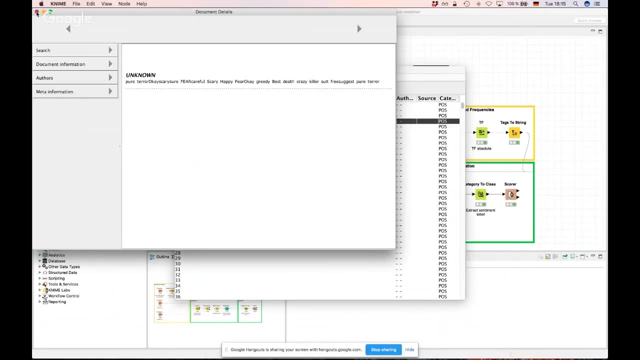 which got either a tag- negative or positive. And if we look now at the document viewer, we actually see that we don't see the index anymore. But if I double click I see now only the words which got tagged, and all the words which didn't get a tag we deleted. 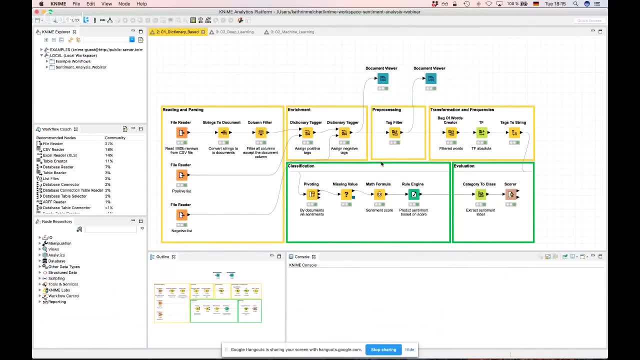 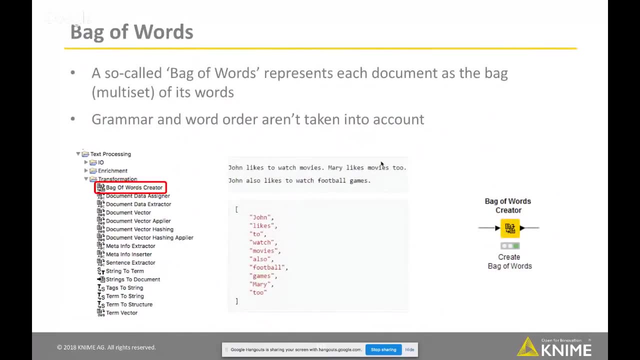 The next step is to create a bag of words. And to explain what a bag of words is, I created another slide. So a bag of words represents each document as the bag, so as the multi-set of the words in the document. But a bag of words doesn't take into account. 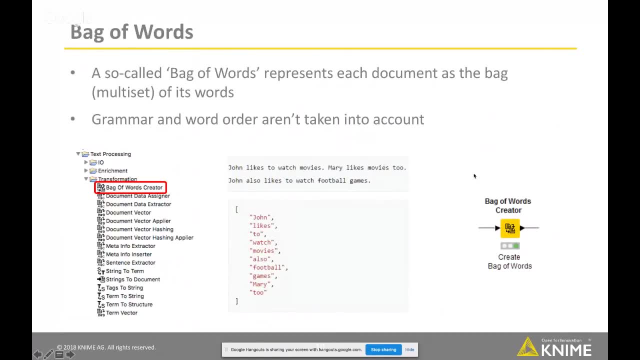 the word order or how often it occurs. So if you look, for example, at the text John likes to watch movies. Mary likes movies too. John also likes to watch football games, then this here would be the bag of words. So we have, for example, the word John occurs. 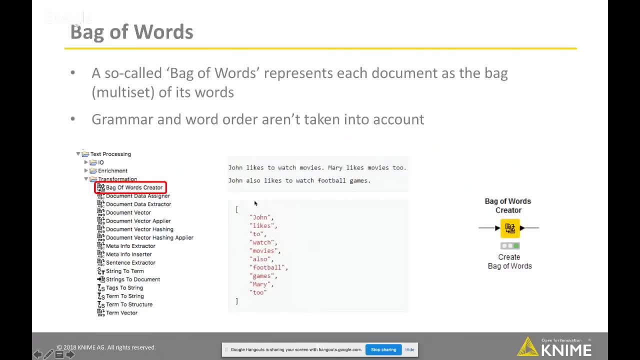 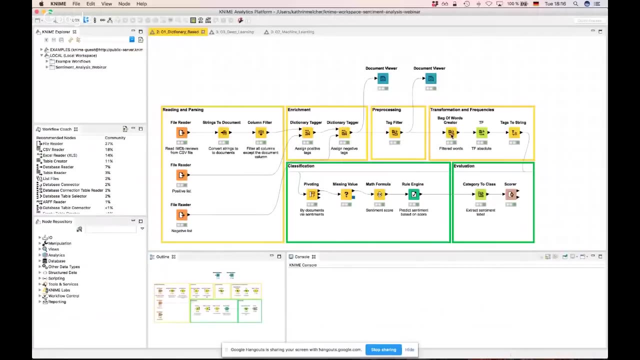 in this document. This is the text, but it is only once in our bag of words, So it's really all the words that occur in the document And if you take a look now at the output of our document, a bag of words. creator. 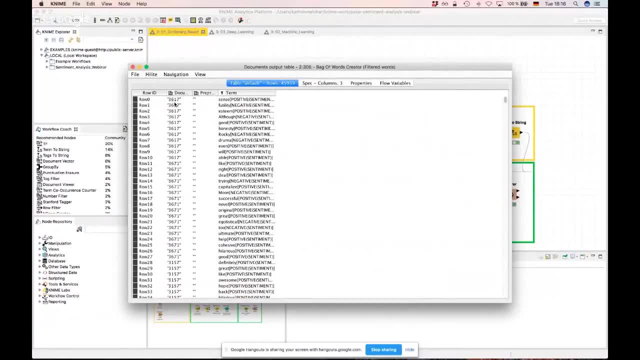 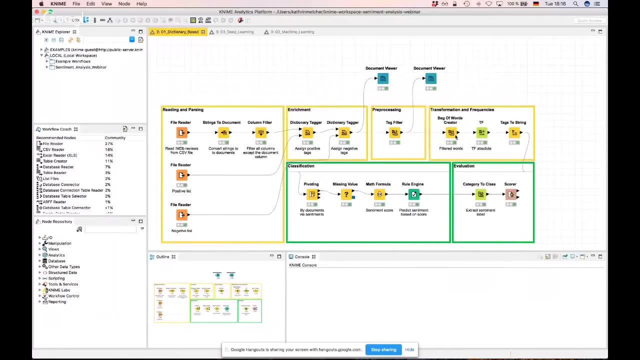 we see here. for each document which we see here on the index, we get all the words which are in this document And in addition also the tag, So whether it's got a positive or a negative tag. But what we don't know yet is how often. 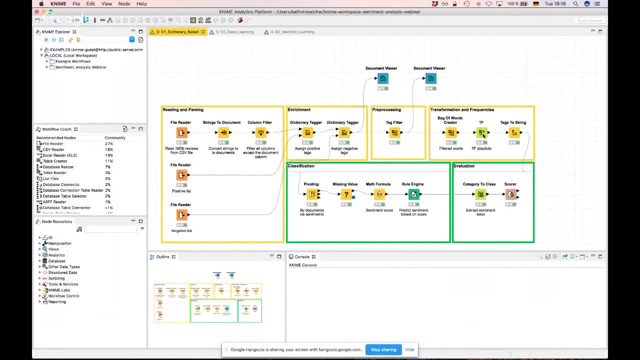 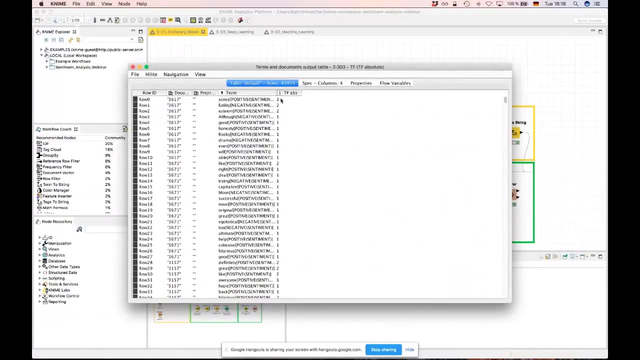 each of these positive or negative words occur in the document And therefore we can use the TF, the term frequency node, and calculate the absolute term frequency for each word. And this node adds now one additional column to our output table, telling us how often each word occurs in the document. 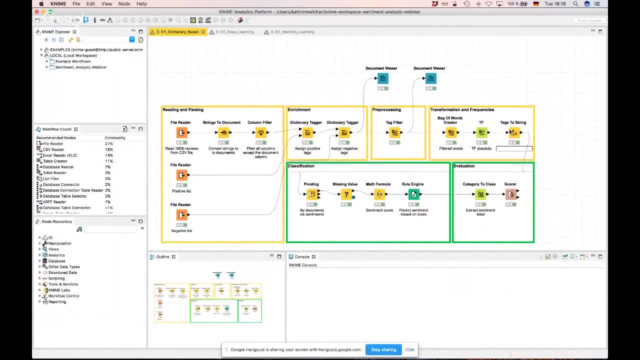 Last, we extract the tag- whether it's positive or negative- into a string So that we can use this information now in the pivoting node to count how many positive words and how many negative words we have in each document. And then we are nearly done. 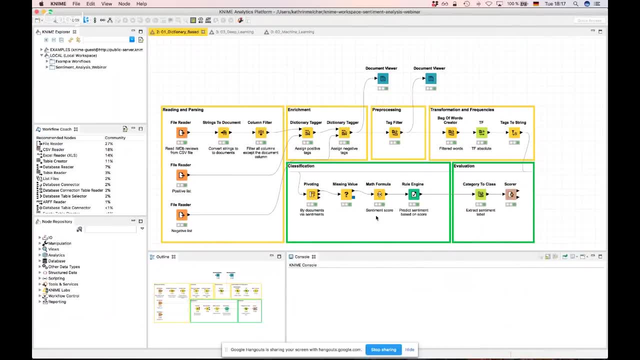 So we can use the math formula node to calculate now the sentiment score which you saw on the slide. So we calculate the number of positive words minus the number of negative words and we divide by the number of words in the document, And then we can use the sentiment score in the rule engine. 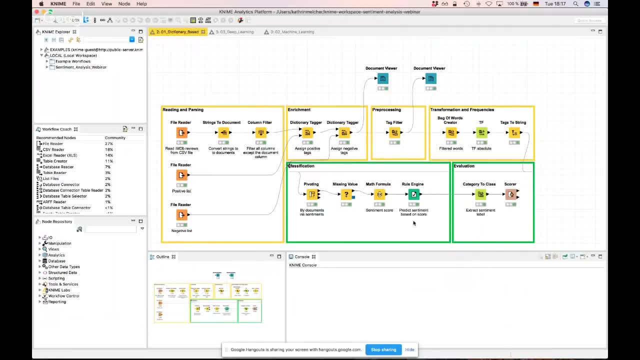 node to actually extract whether it's a positive or a negative. And, last, I said, we want to also evaluate, of course, how good our rule-based approach worked And therefore we need now the true class information, And the true class information is something that we added. 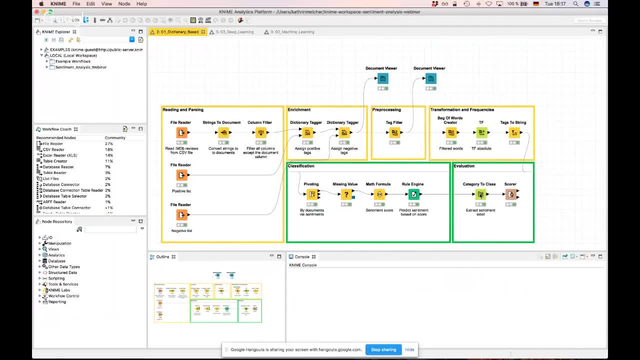 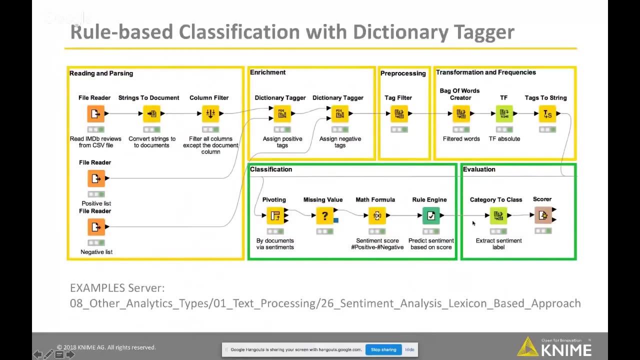 here in the strings to document node, to our document cell, And we can now extract this information again with the category to class node and then evaluate the performance of our rule-based approach. You can find this workflow, which I just presented, on our public example server. 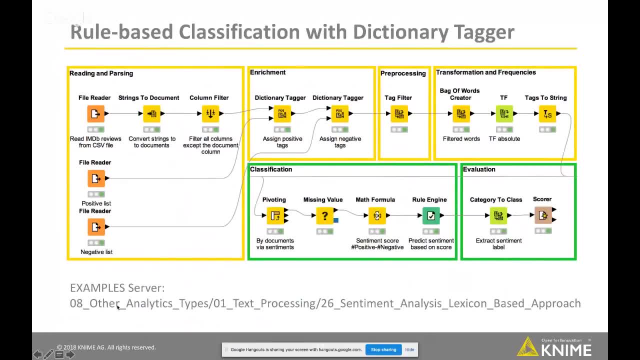 under this following link or in the following folder. So it's other analytics types: text processing and then sentiment analysis, lexicon-based approach. But the slides will be available later as well, So you can also look this link up later. This was now the lexicon or the rule-based approach. 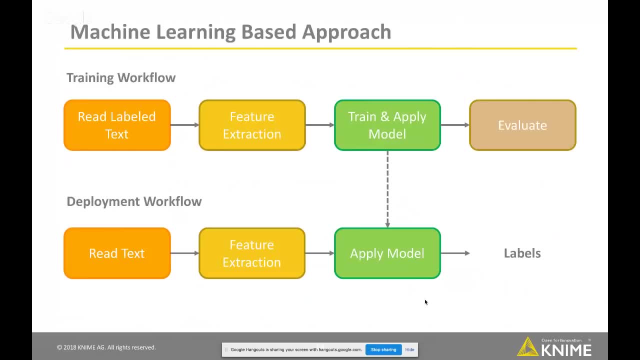 And the second approach is the machine-based approach. This is a machine learning-based approach where we want to use a supervised learning algorithm. When we want to use a supervised learning algorithm, we normally have two workflows: We have a training workflow and then we have a deployment workflow. 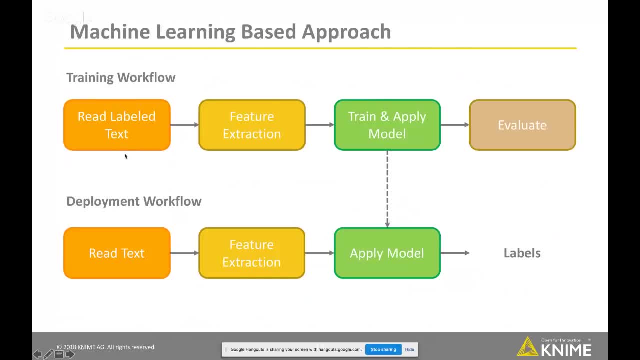 In the training workflow we read our labeled texts. So here we really need labeled text. So we need someone to manually label some of the values in advance so we can train an algorithm later. This is a big advantage actually of the dictionary-based approach. 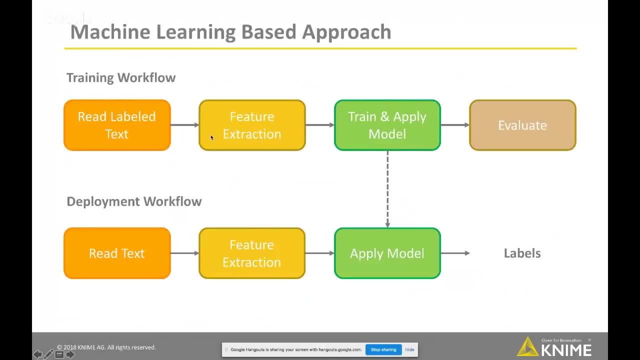 because there you don't need labeled data and it's often hard to get labeled data- And once you have your labeled data, you can do some feature extraction and then train a model where you create a training and a test set so you can train and apply the model. 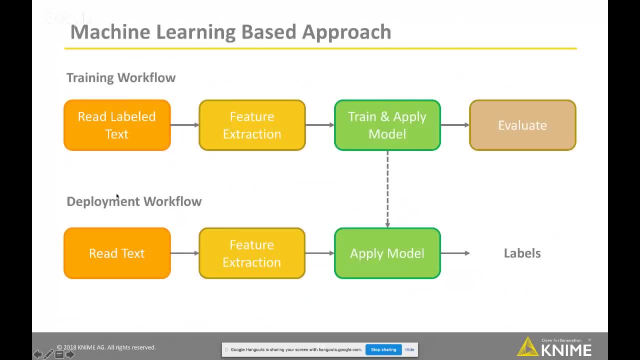 and evaluate your model, And once you're happy with your model, you can then actually build a deployment workflow which you can use then in production. where you read in new text or new reviews where the label is unknown, You do the same feature extraction. 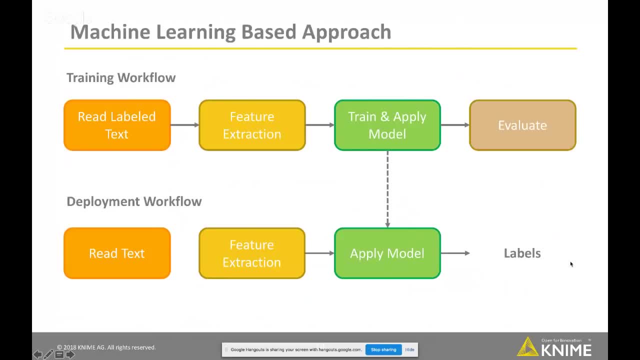 like in a training workflow, then you can apply your model and then you get some labels, And depending on which model you want to use here, you also use different feature extraction. So the feature space looks often different depending on the model you want to train. 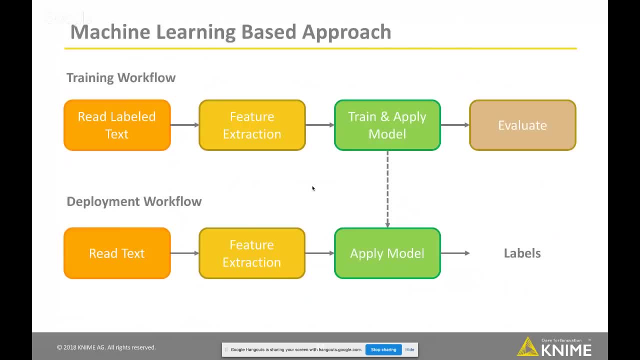 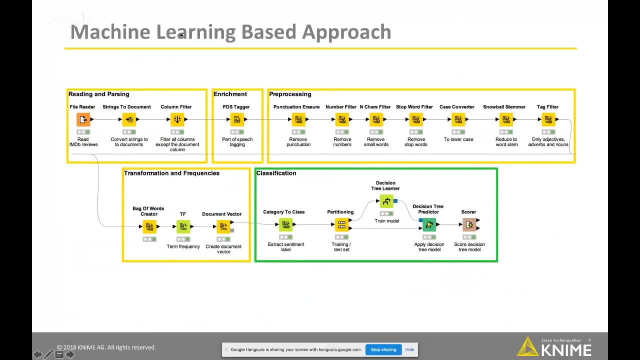 especially if we compare between a kind of classic machine or supervised learning algorithms and deep learning. We now first want to focus on the machine learning-based approach, where we use some classic supervised learning algorithm like the decision tree, And here the first steps are actually really similar. 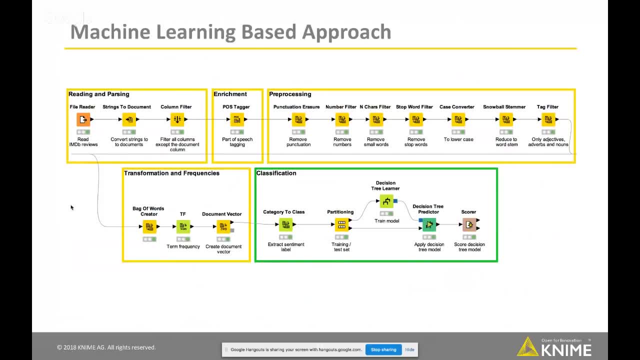 to what we've seen in the lexicon-based approach. We again read in our files and create our document cell and then delete all the columns which we don't need anymore because we have the information in the document cell, And then we assign here another tag type. 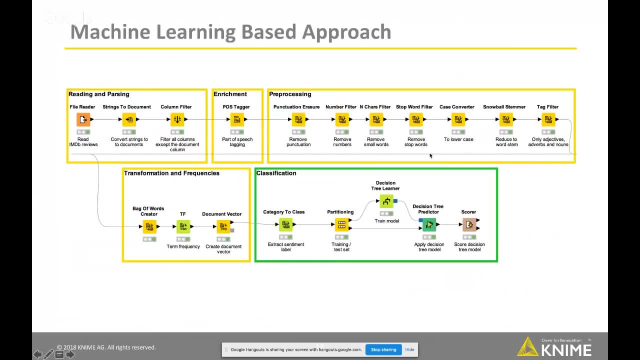 so here we do a part of speech tagging and then we do a number of pre-processing processing steps where we delete words which are not important or tokens which are not important or which we don't want to take into account in our analysis. 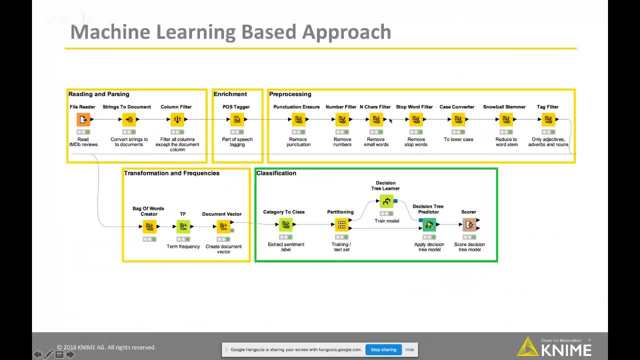 This is, for example, punctuation, which we remove, or small words with the end-chars filter, So we can say we remove all words that have less than three characters. or we can use the tag filter again and this time use the information. 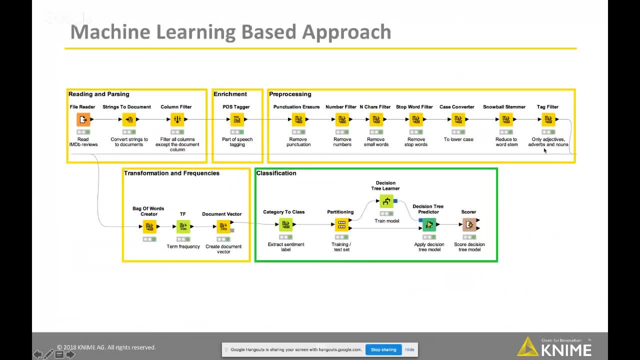 which we got from the part of speech tagging, that we only want to use adjectives, adverbs and nouns. Then we create again a bag of words and can assign a term frequency, And then the next step is to create a document vector. 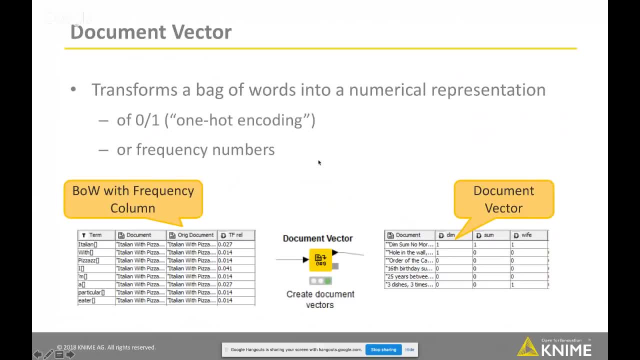 And the document vector transforms a bag of words into a numerical representation. And here we get a numerical representation for each document And already in the document vector we have two different options. So in general, what is a document vector? In the document vector we have for each word. 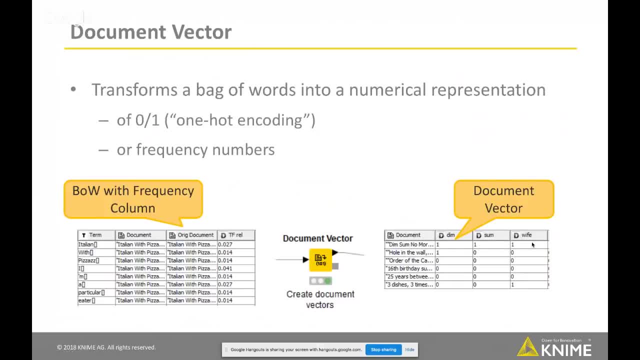 that occurs at least in one of the documents. after all the pre-processing steps, we get one column And then if we have a zero, one hot encoding. we have a one if this word occurs in a document and a zero if it doesn't occur in a document. 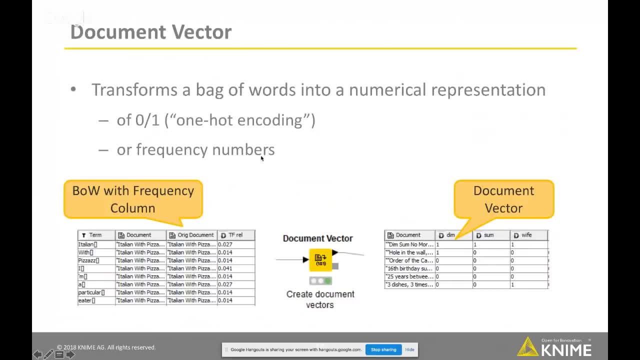 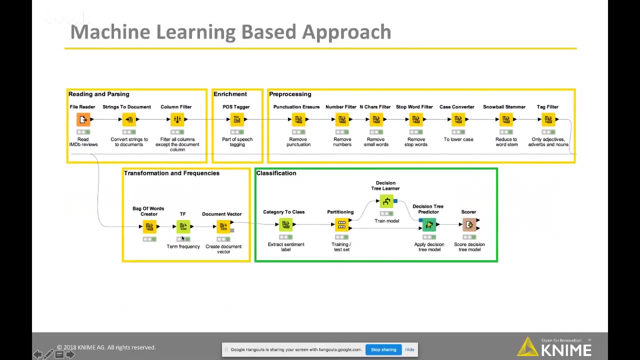 Or we can also have a document vector based on frequency numbers, And then we wouldn't have here only zeros and one, but also how often this word occurs in each document. And this is what we do here: We take our bag of words and list the term frequencies. 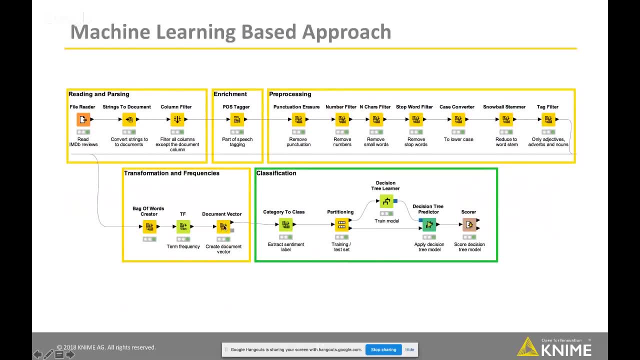 and then create a document vector for each document so that we know which of the words that occur in one of the documents occurs also in a special document. And then again we need again our class label, So we extract our sentiment label And then we have now our numerical representation. 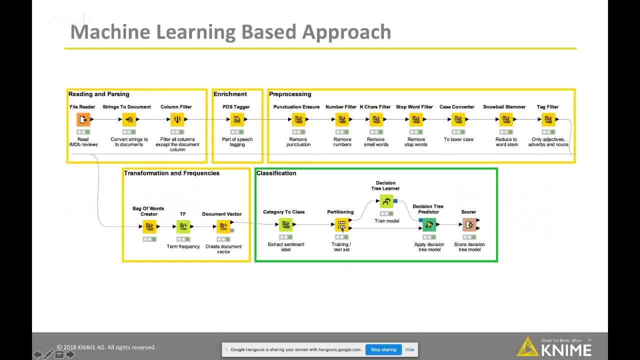 with our label. So we are now in the situation that we can use the normal KNIME nodes, And what we do here is we create a training in the test set And then, on the training set, we train a decision tree And then we use the predictor note. 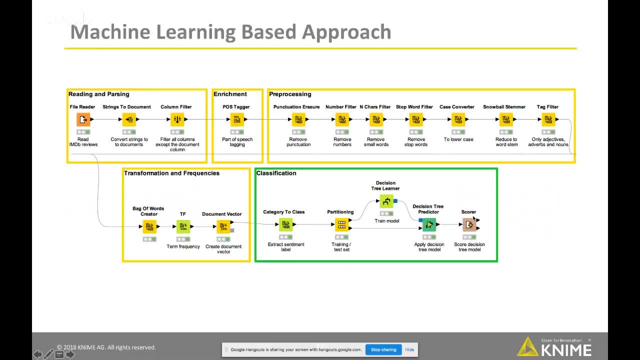 to actually apply the decision tree to the test set And then we can evaluate the model. This decision tree, learner predictor. this is something that we have for all our training or all our learner nodes, which we call the learner predictor mode. So instead of using here, we can do this model model. 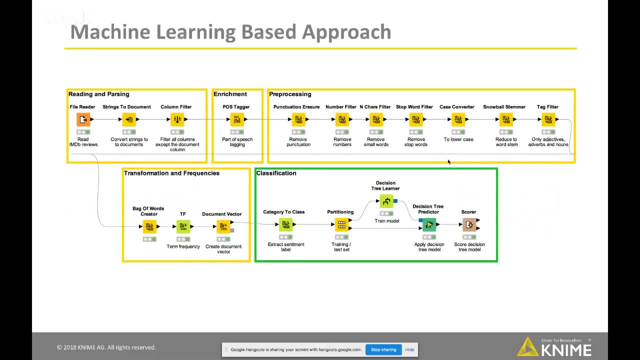 So instead of using- here we can do this model model, the decision tree learner, we could have used also a tree ensemble learner or gradient boosted tree learner. Also for this example, we have a similar workflow on the example server and which you find on 0.8 other analytic types. 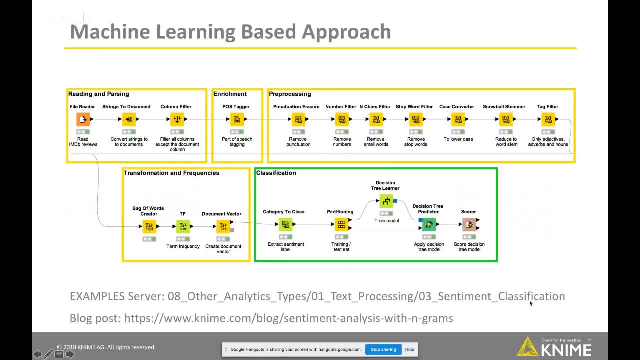 0.1- text processing and then 0.3 sentiment classification. And here you will. if you open this workflow, you will see that it uses here a slightly different pre-processing steps. So depending on the text you are reading in. 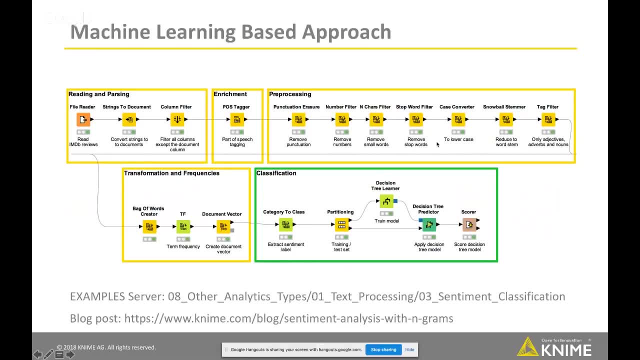 you could use here also more cleaning up or less cleaning up. but remember: each word that in the end is still in one of your documents becomes then one column in your document vector, So your feature space there can get really big. In addition, we have also a blog post. 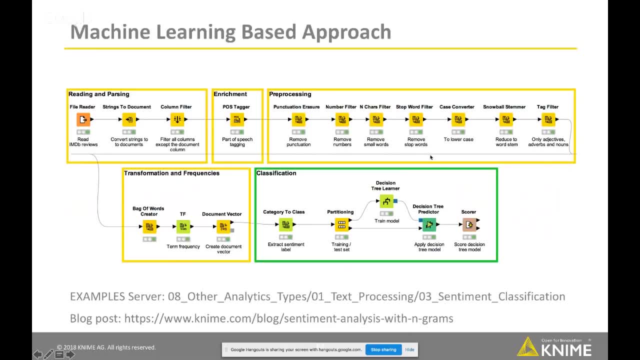 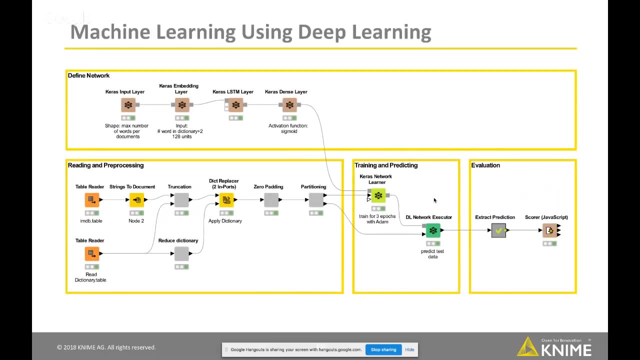 on sentiment analysis with Ngrams. Here we create Ngrams in the pre-processing, and this blog post shows how you can improve your model by using Ngrams instead of only one grams. Next we come to the second example of the machine learning based approach. 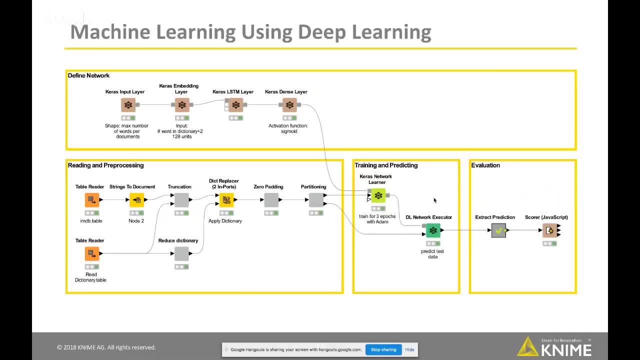 And here we want to use the Keras integration or the deep learning integration in life. And what we do here is we define a network, We have again some reading and pre-processing steps and then we can train the network with the Keras network learner node. 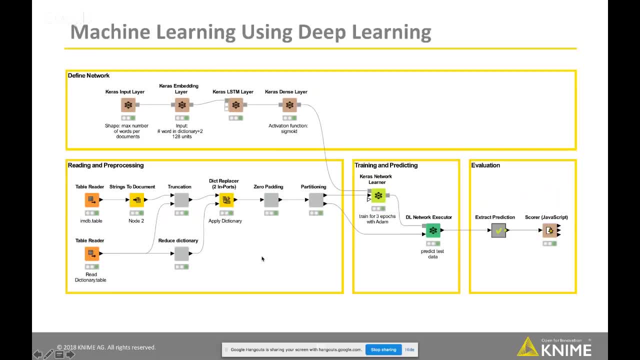 and then apply it and also evaluate the model. But, as I said in the beginning, the pre-processing is not always the same And actually it is in this case really different because we want to use the network we define. here is a recurrent neural network because of this LSTM layer. 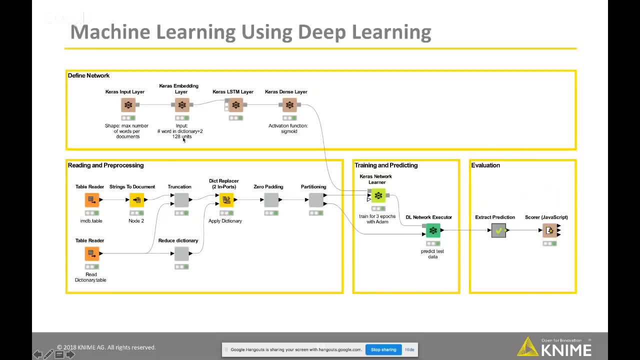 And this has the advantage that we take into account the word order. Remember, when we created this bag of words, we lost the word order. but also in the beginning we said that alike can become negative if there is a notch in front of it. 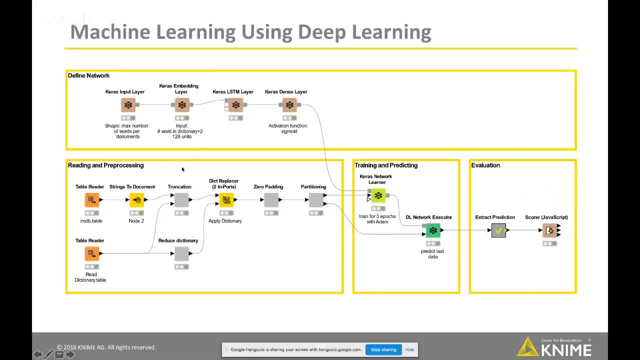 So not like So. therefore, the reading and pre-processing is also different And before I talk about the network structure I used and the learning, I want to focus for a second or a minute on the reading and pre-processing part. So again, of course, 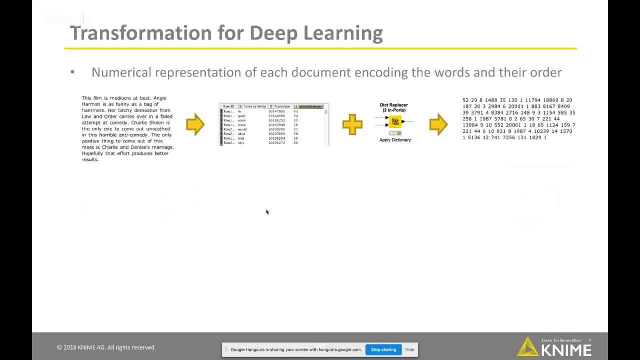 we need a numerical representation for each document, But, as I said, this time we want to take into account also the word order, And what we do here is So, if we have a text like here on the left, we can use a dictionary where we assign to each word an index and then apply this dictionary. 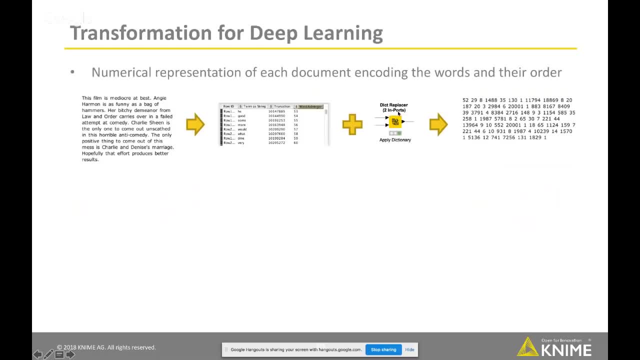 For example, in line with the dictionary, the placer node with two input ports, And then we have only a sequence of numbers afterwards. A second requirement for learning neural networks is that the input shape in one batch size has to be the same, And therefore we want to have each document in the same size. 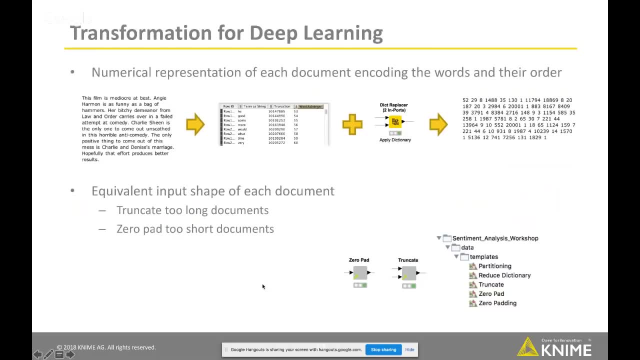 And as each word in the document becomes one number, this means that we have to define a maximum number of words which we want to take into account of each document, And if a document has more words than this maximum number of words, then we have to truncate it. 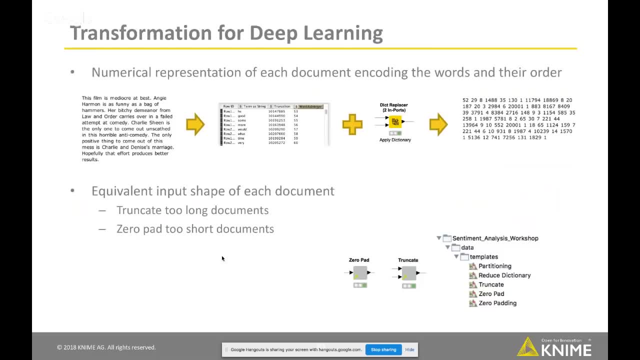 This means we just cut it off, And if it has less numbers then we have to zero pad this document. This means we just add zeros. And for those two tasks I created two rep metanodes and saved them as templates so that you can see them in the KNIME Explorer. 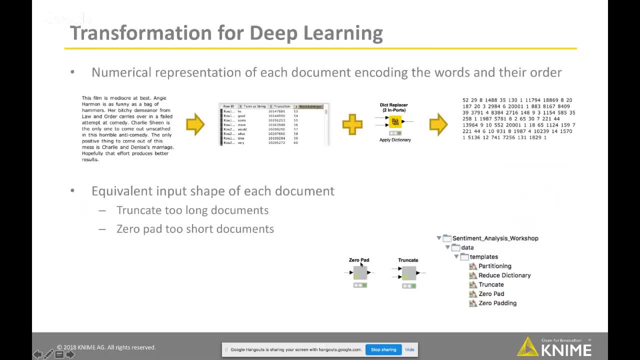 For those of you who don't know what rep metanodes are, we have in KNIME the option to actually hide some of the nodes inside of a rep of a metanode to organize and structure your workflow, And this is what I did with the zero pad and truncation nodes. 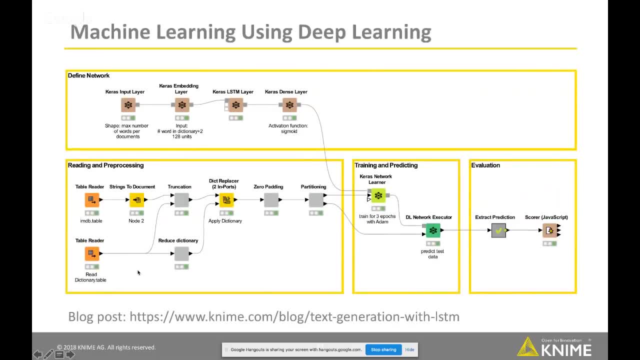 So if you look now into the reading and preprocessing part, we read in the documents again the reviews, we create our documents and we read in addition the dictionary. Then the first thing we do is we truncate two long documents with the truncation metanode I created or I prepared. 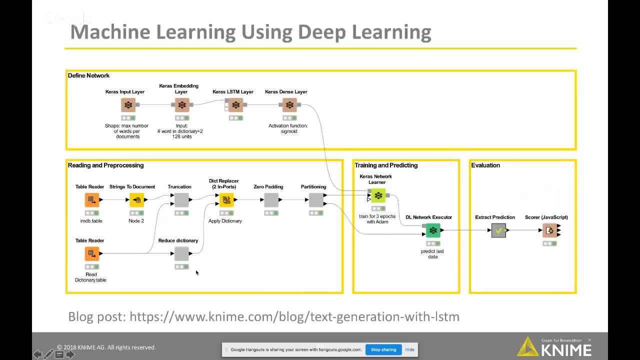 And then, in addition, we don't say that each word in the document gets its own index, but, for example, only the 25,000 words, which most often get their own index, And all the other words in between we just index in code with the default value. 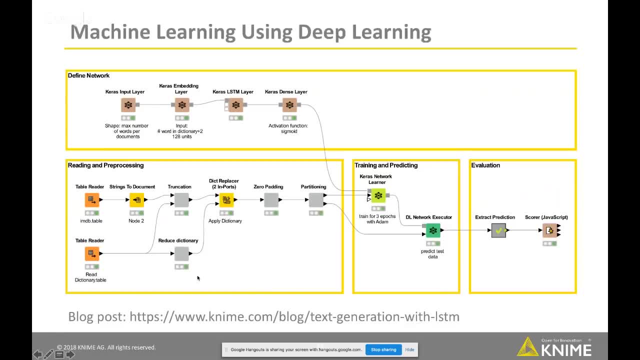 And therefore we create a reduced dictionary where we decide how many words we want to take into account, Then we apply this to our documents, and then the zero pad, and then we are ready with the reading and preprocessing part. Next we have to define the network we want to learn. 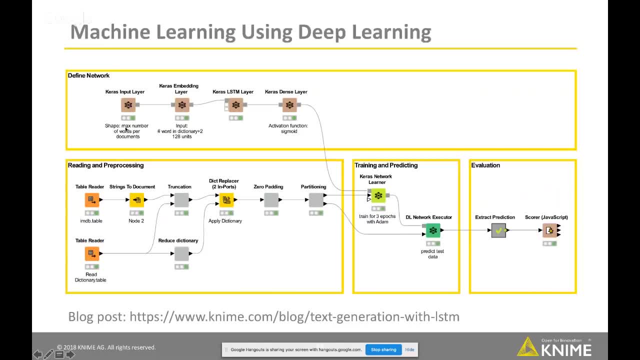 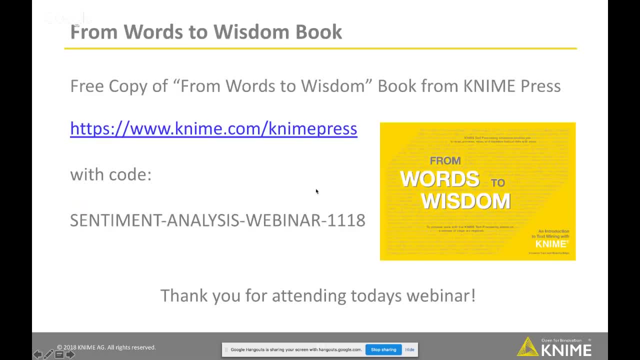 And this brings us to the end of our today's webinar. As a little thank you, I have a promotion code for you for our book From Words to Wisdom, which is an introduction to text mining with KNIME. So if you use the promotion code sentimentanalysiswebinar1118,, you can get a free copy of this book. 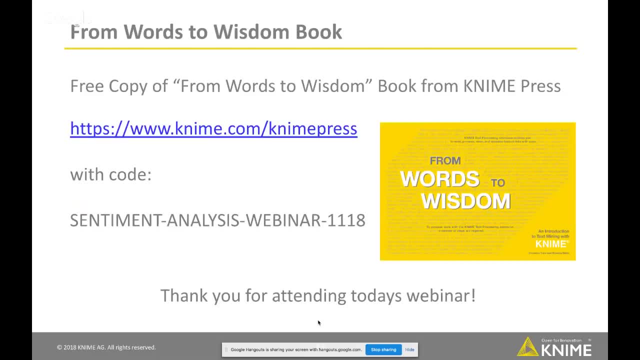 And this brings us to the end. Thank you for joining today, And I think that's it. Have you got some questions while I was talking? Yeah, so we are not at the end, So we have a few questions, OK. the first one here is about text vectorization. 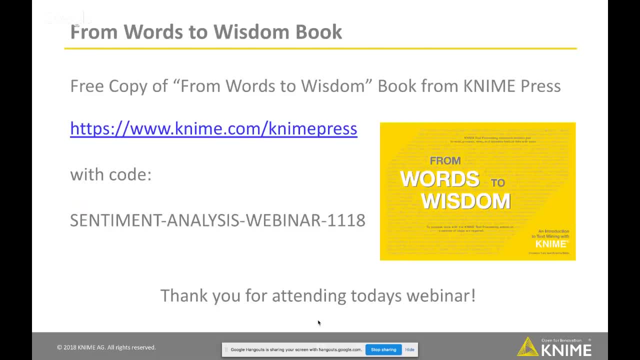 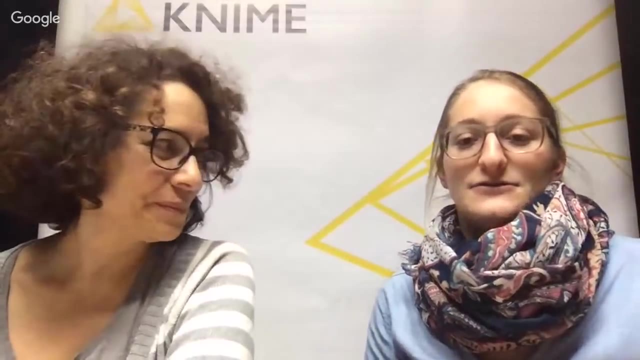 So they say text vectorization can produce high dimensional data sets. Is there a way to reduce the dimensionality of the large data sets where each column is a word? I think I will stop sharing the screen also. Yeah, so there are different things that you can do. 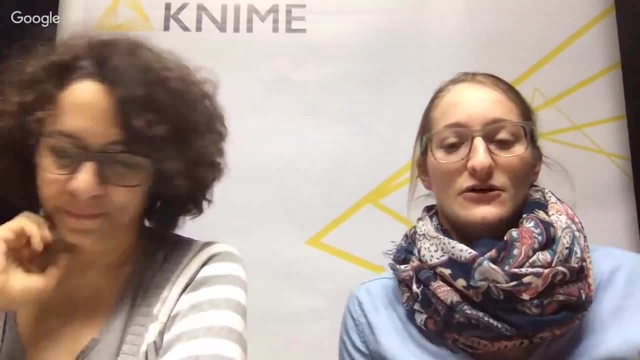 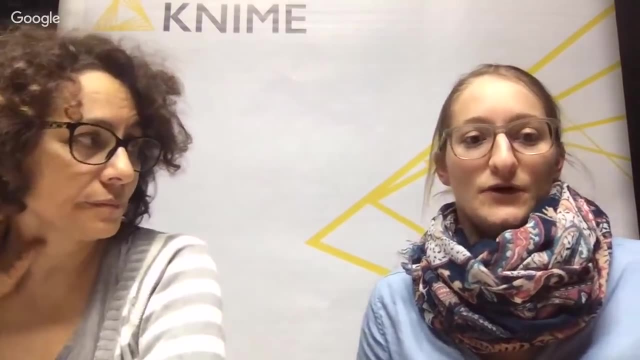 One is, for example, we saw in the machine learning based approach all this cleaning up And I said there is another workflow available on the example server. There we decided to use only the words that occur in many documents. So this is another thing that you can do: that you clean up more. 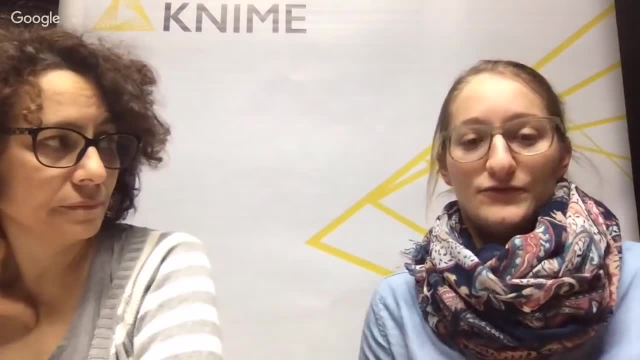 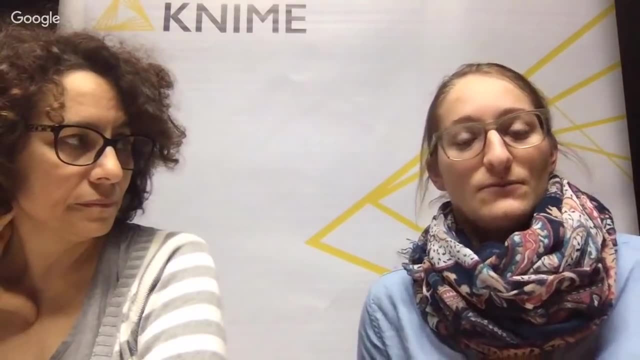 In the pre-processing, you delete more of the words. Another thing that you can do is to use these embedding layers or use one of the pre-trained embeddings from Google, like Word2Vec or Globby, where you get a better representation, Where you get a better representation for each word. 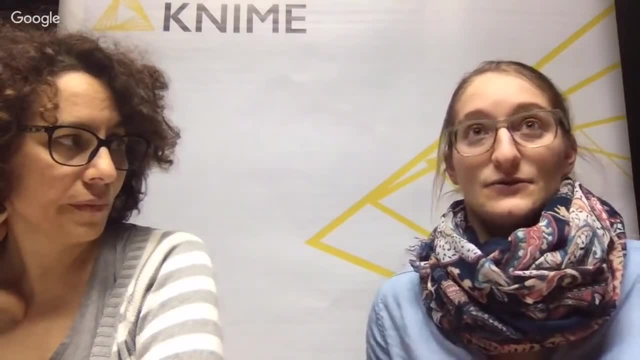 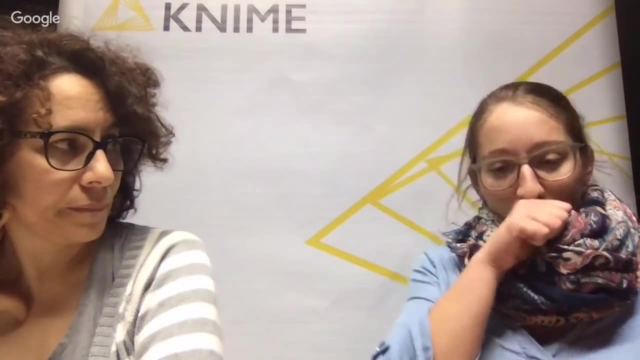 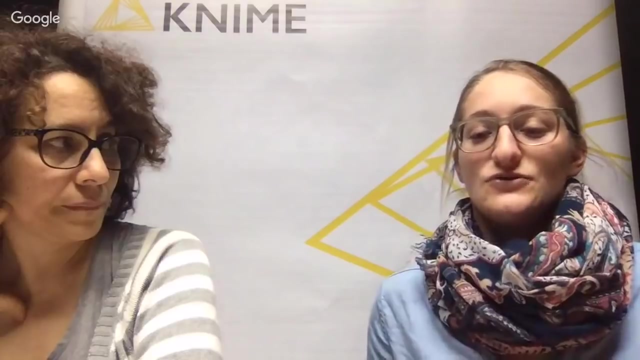 And therefore you need maybe less. So it becomes smaller the feature space. And the other thing that you can do is you can use keyword extraction, But there you should be careful that you don't delete too much information if you say you want to have only three or four keywords per document. 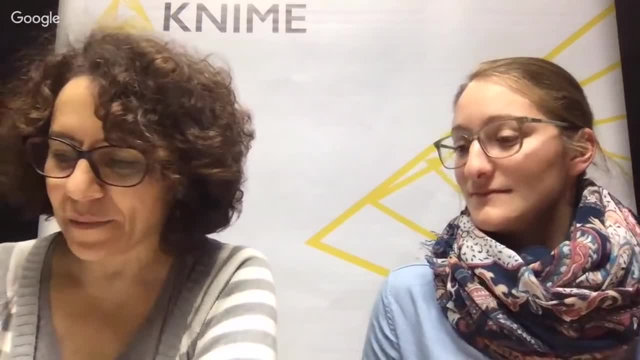 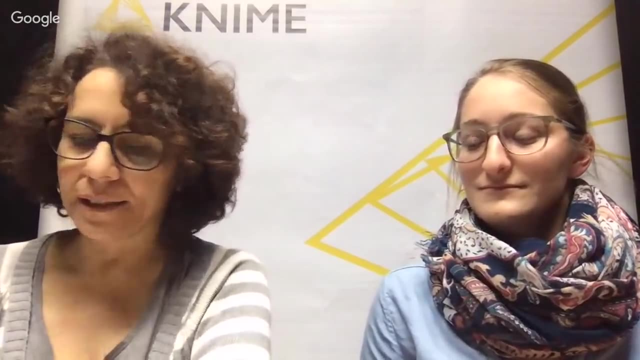 OK. Second question: is you use the part of speech node, So the part of speech tagger node? Why do I need it? I mean I have to. He says he has to only to tag by sentiment. So why part of speech? 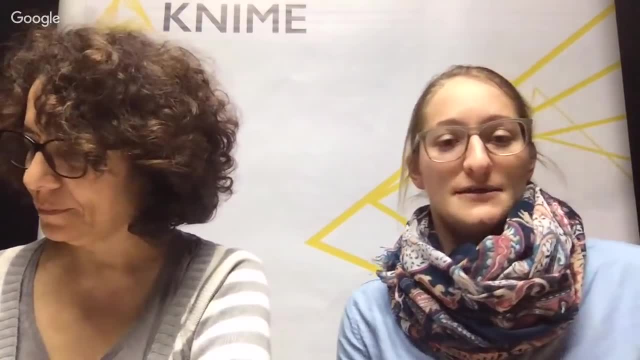 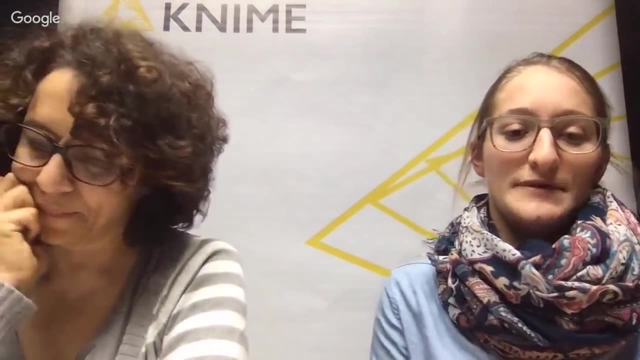 So we use the part of speech tagger node in the machine learning based approach to the pre-processing Because we did afterwards with the tag filter node some filtering based on the part of speech tags. And why does this make sense? If you remember in the beginning, 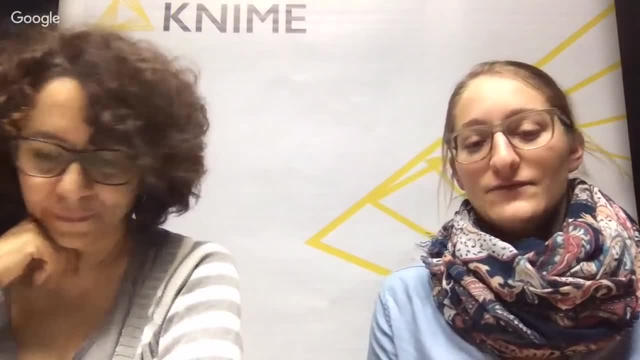 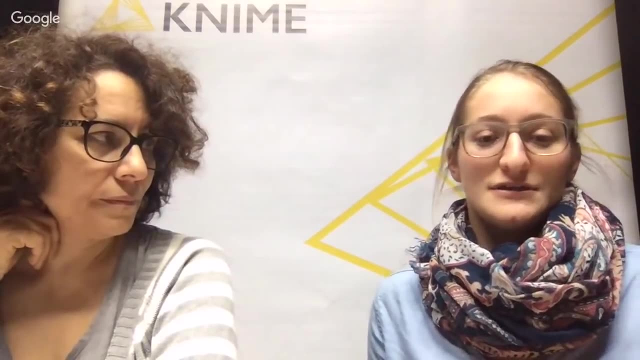 I had the example with the different loads, And like was in some places a verb But in the end also a preposition, And if it is a preposition then the like is not as important as it is if it is a verb. 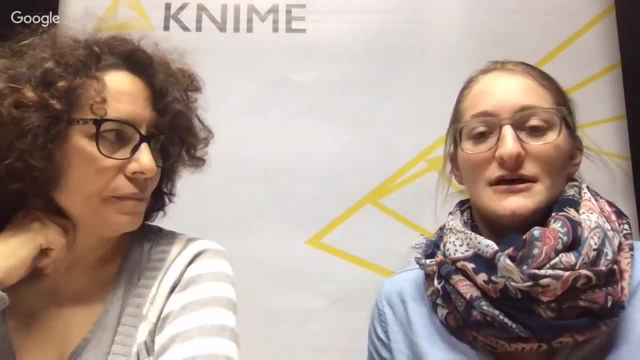 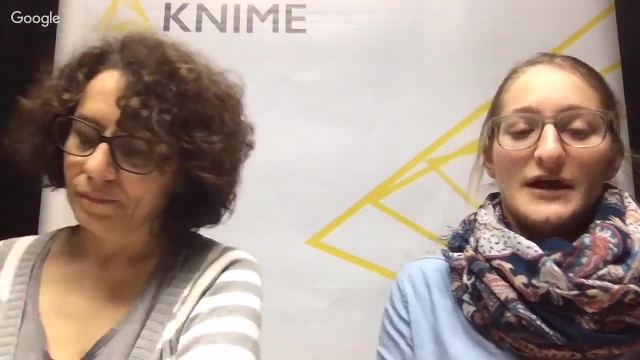 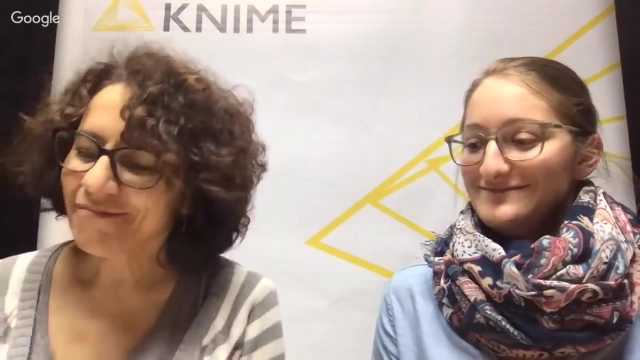 And that's where the part of speech tagging is in the first place helpful, so that you can then delete or decide which words you want to have in your analysis based on these tags. So next question is: He's about sarcasm And idiomatics. 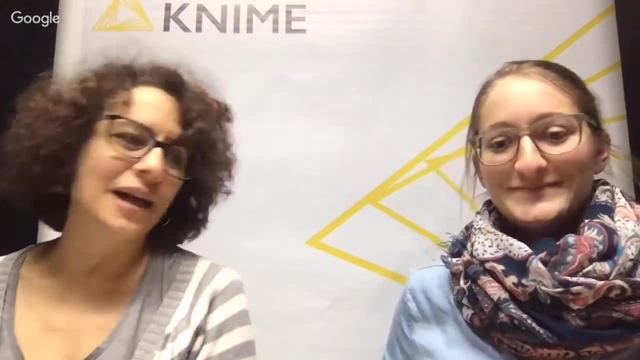 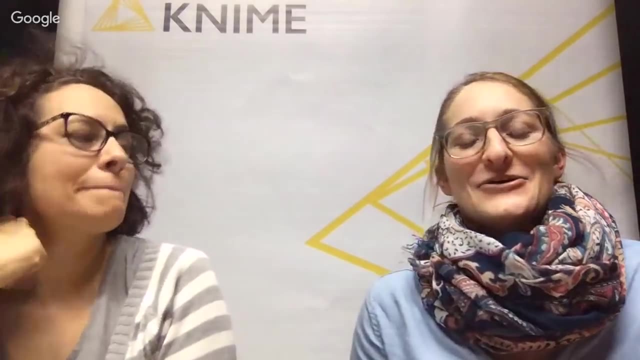 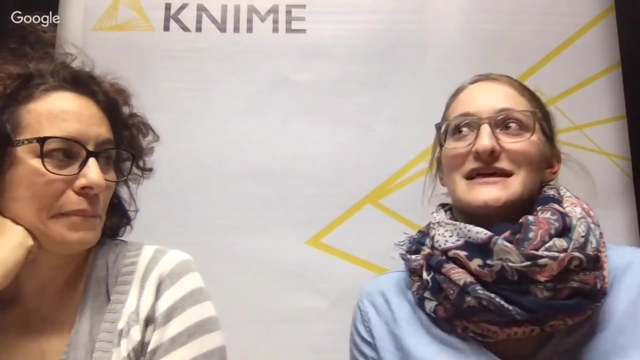 How are sarcasm and idiomatics taken into account? Yeah, that's a hard one, And I think So The last time someone else asked me this question before and I said I think it's not possible that you take that you find out sarcasm if you have only text. 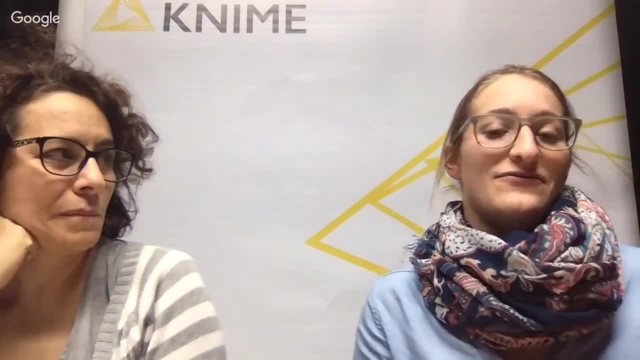 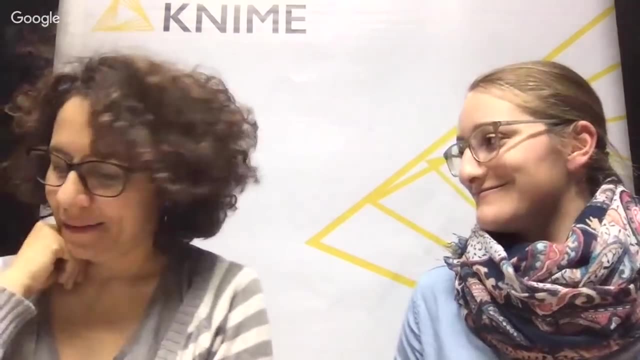 But maybe if you have audio files then you maybe can find out the cousin already, or But I think it's. I'm not sure whether it's possible or not And I never tried it. Yeah, I don't know whether you have a better. 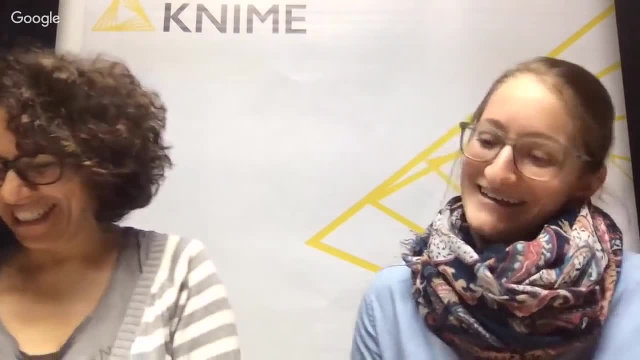 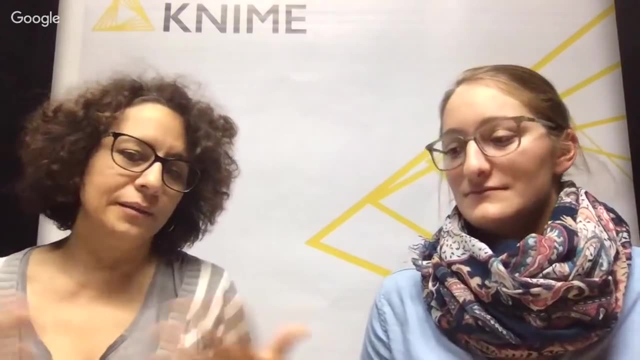 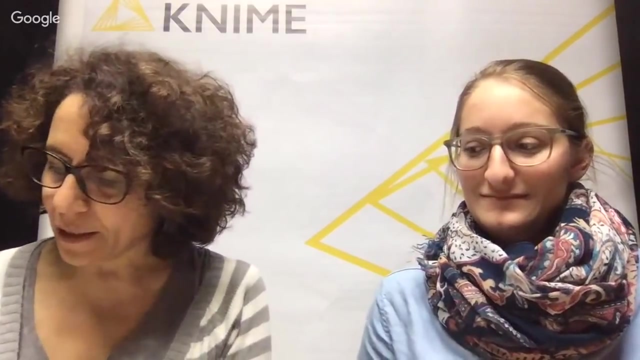 No, Sarcasm is also hard for humans, That's true. But idiomatic expressions, idiomatic expressions. you can still take together, Right, And build a dictionary of idioms and and then take them. that you can do. And then the third question. 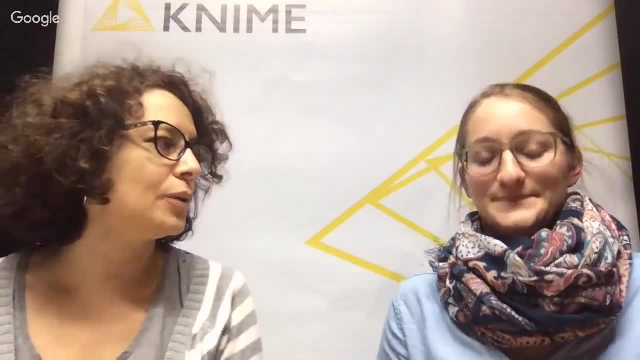 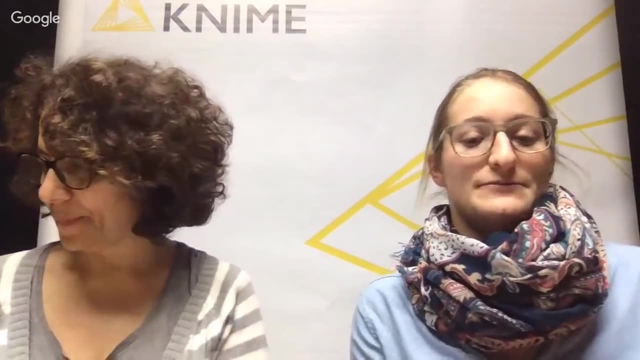 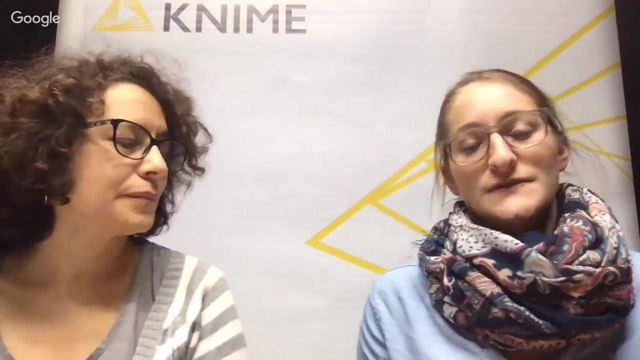 What does the embedding layer do in a neural network? So, as I said, embedding layer extracts a better representation for each word by taking into account the surroundings of which words are around this world, And then words with a similar meaning get a similar vector. 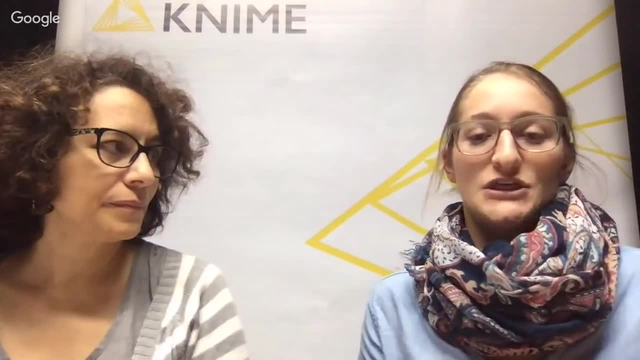 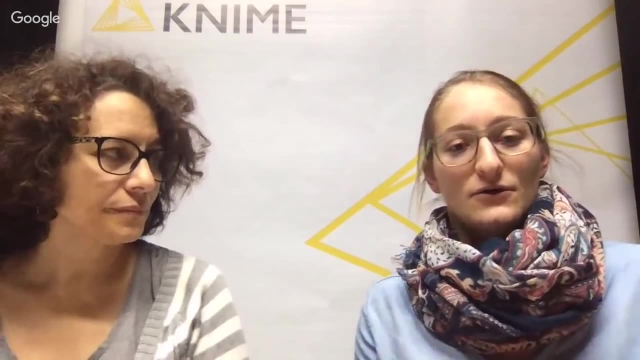 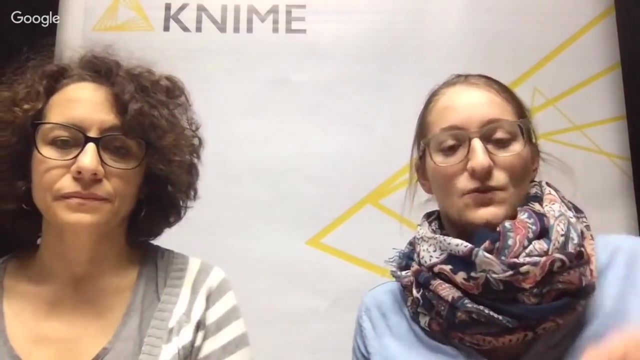 So you just get a better representation for each word and therefore also a smaller one, Because, for example, normally you, if you have a zero, one hot encoding for each word, you have always the dictionary size And then at some point One, that which says this is this word. 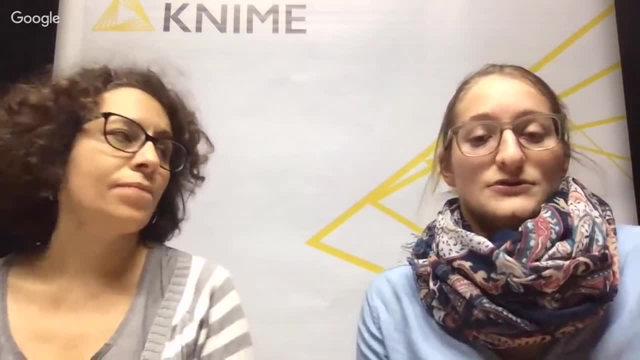 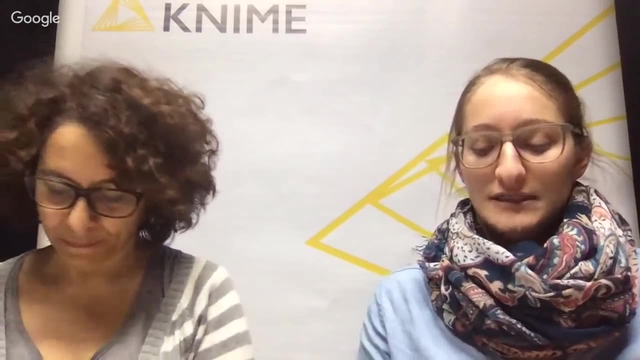 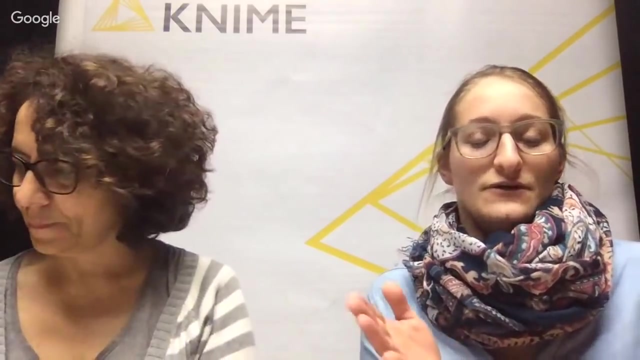 But with an embedding layer. you would have, for example, an output dimension of 100. So you would have a vector representation for each word with of dimension 100. And then words with a similar meaning would have a vector representation which is close to it. 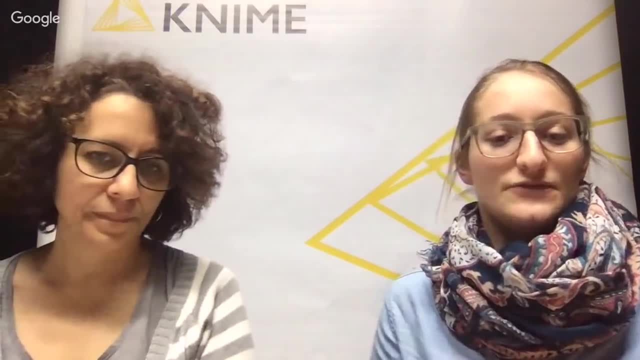 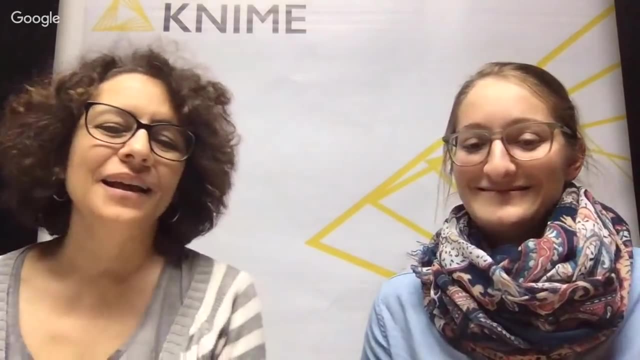 And words with different meanings have completely different vectors. OK, I have no more questions. So, unless something comes in in the last minute, I thank you all for attending this webinar and I hope to see you at the next nine webinar. Bye, Thank you. Bye, bye.